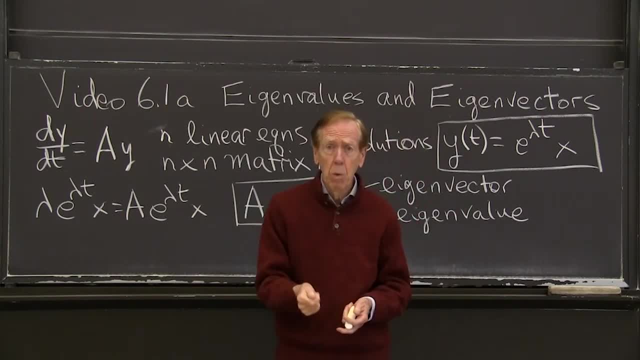 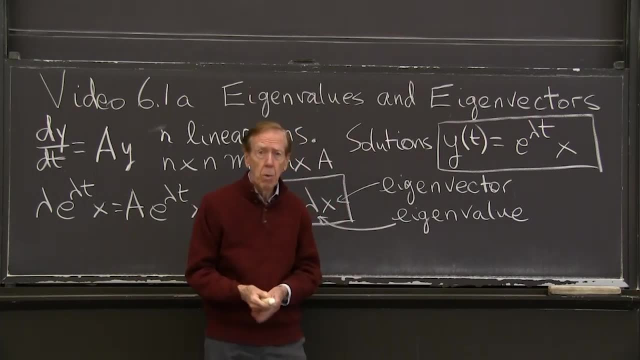 Good, And now I can tell you right away where eigenvalues and eigenvectors pay off. They come into the solution. We look for solutions, We look for solutions. We look for solutions of that kind. When we had one equation, we looked for solutions, just e. 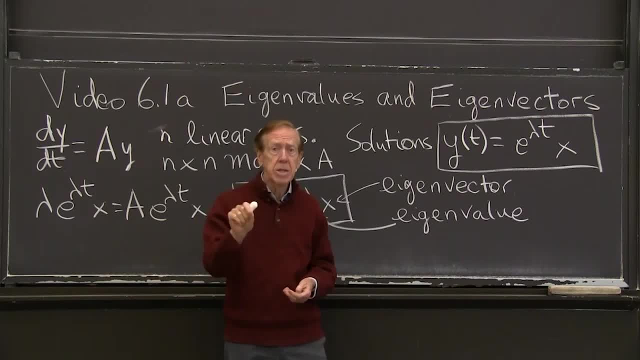 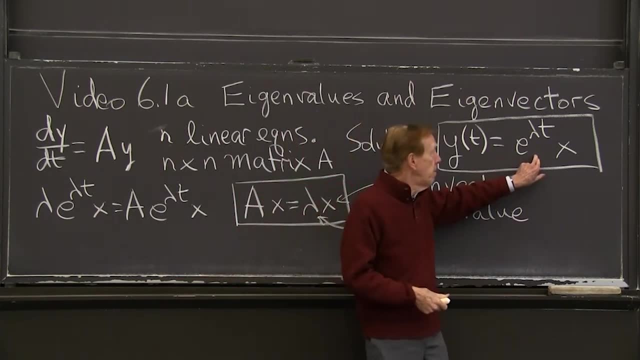 to the st And we found that number s. Now we have e to the lambda t. We changed s to lambda, no problem, But multiplied by a vector, because our unknown is a vector. This is a vector, But that does not depend on time. 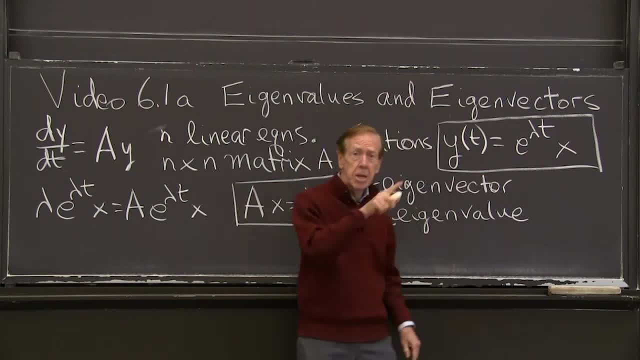 That's the beauty of it. All the time, dependence is in the exponent Exponential, as always, And x is just multiples of that exponential, as you'll see. OK, So I look for solutions like that. I plug that into the differential equation. 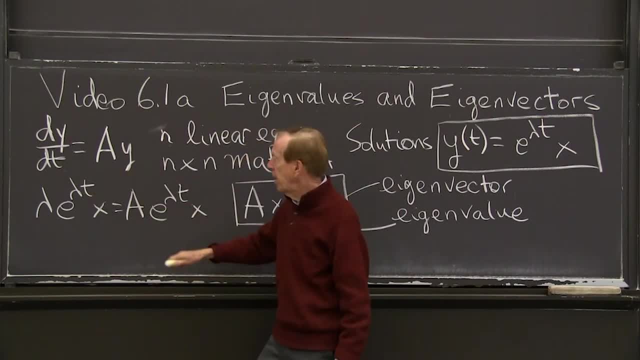 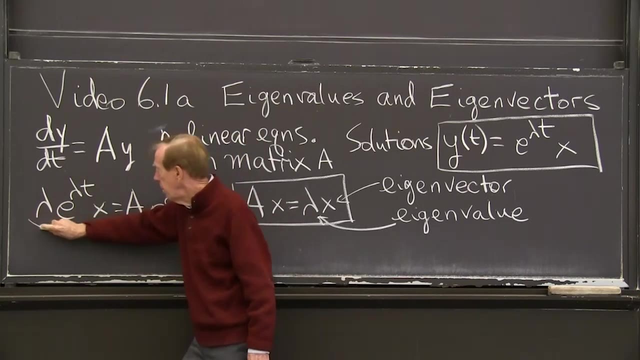 And what happens. So here's my equation: I'm plugging in e to the lambda tx. That's y, That's a times y there. Now the derivative of y, the time derivative, brings down a lambda. So to get the derivative, I include the lambda. 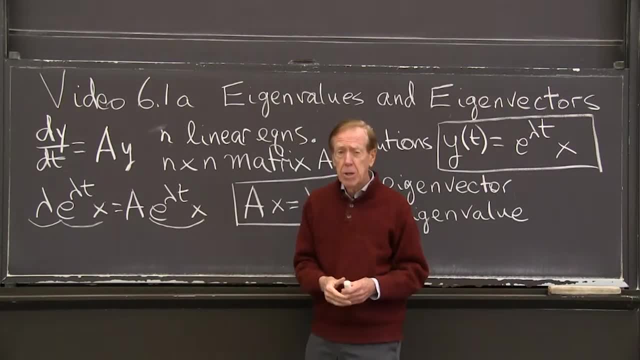 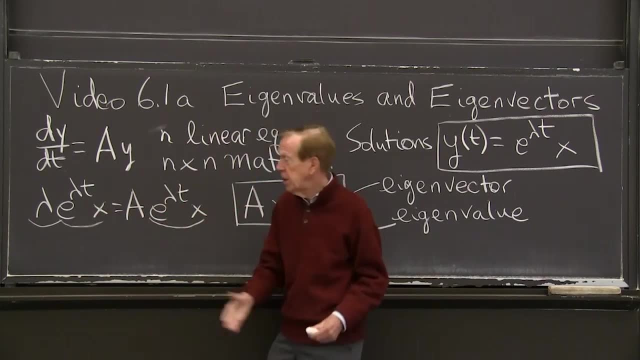 So do you see that substituting into the equation with this nice notation is just. this has to be true. My equation changed to that form. OK, Now I cancel e to the lambda t, just the way I was always canceling e to the st. 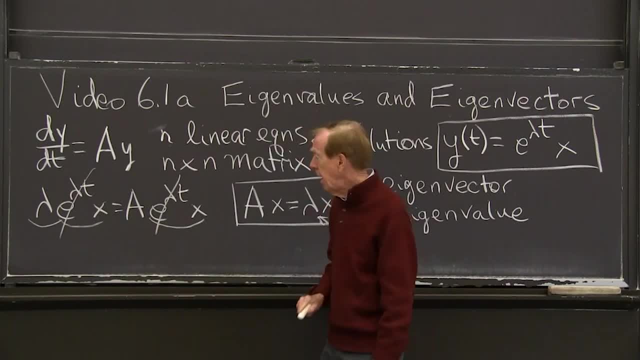 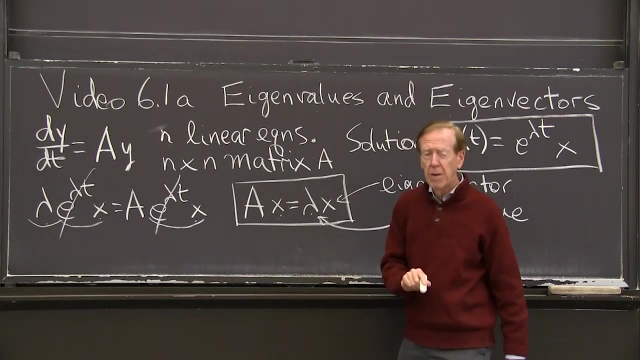 So I cancel e to the lambda t, Because it's never 0. And I have the big equation: Ax, the matrix times my eigenvector, is equal to lambda x. The number, the eigenvalue times the eigenvector. 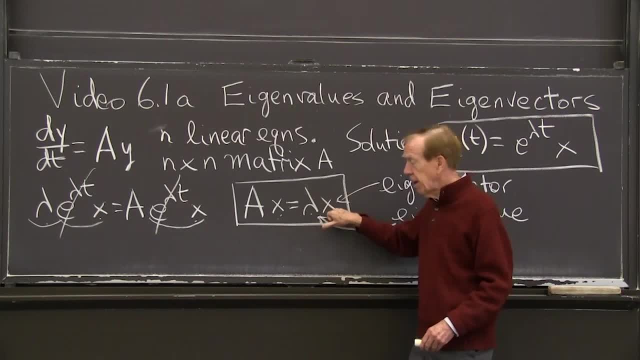 Not linear notice. Two unknowns here that are multiplied A number lambda times a: vector x. So what am I looking for? I'm looking for vectors x, The eigenvectors, So that multiplying by a, multiplying a times x. 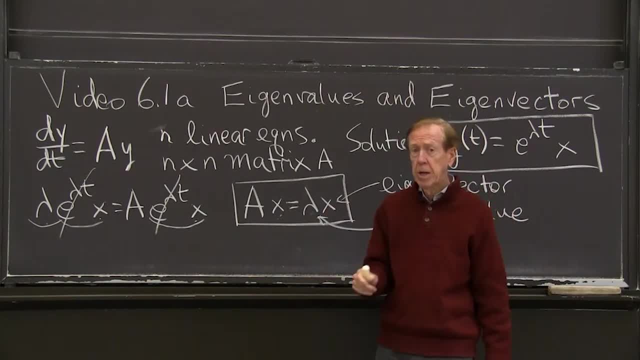 gives a number times x. It's in the same direction as x, just the length is changed. Well, if lambda was 1, I would have ax equal x. That's allowed. If lambda is 0, I would have ax equals 0.. 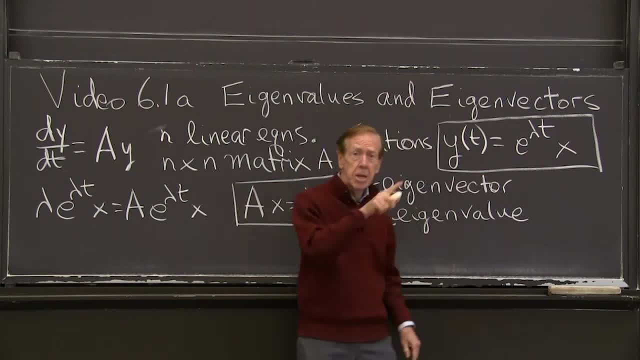 That's the beauty of it. All the time, dependence is in the exponent. It's exponential, as always, And x is just multiples of that exponential, as you'll see. OK, So I look for solutions like that. I plug that into the differential equation. 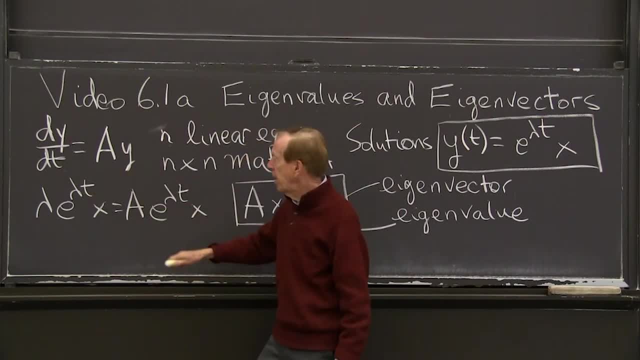 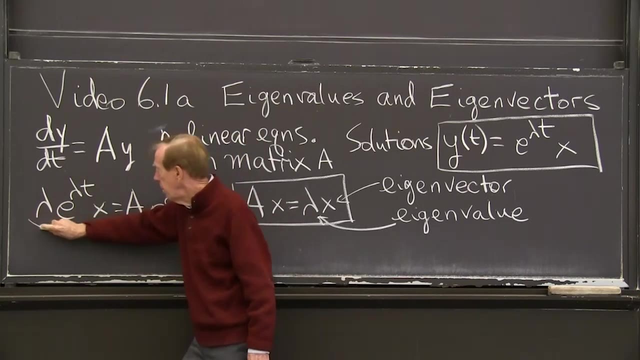 And what happens. So here's my equation: I'm plugging in e to the lambda tx. That's y, That's a times y there. Now the derivative of y, the time derivative, brings down a lambda. So to get the derivative, I include the lambda. 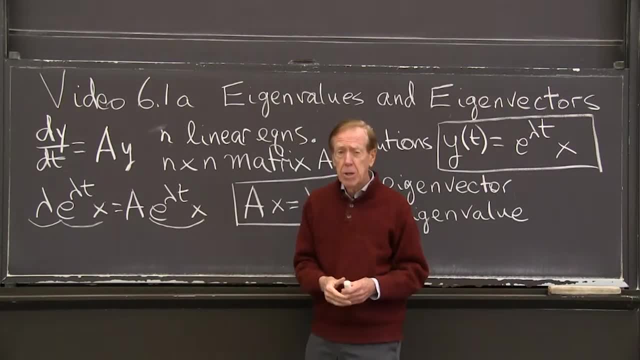 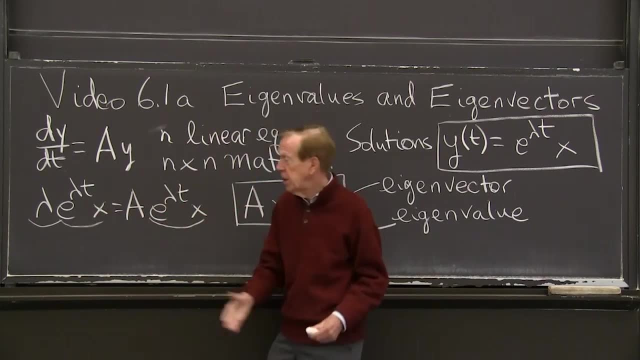 So do you see that substituting into the equation with this nice notation is just. this has to be true. My equation changed to that form. OK, Now I cancel e to the lambda t, just the way I was always canceling e to the st. 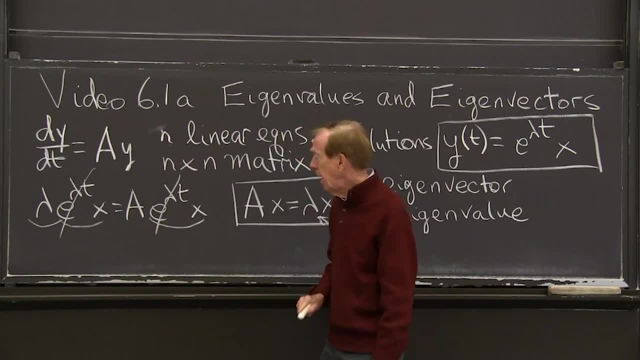 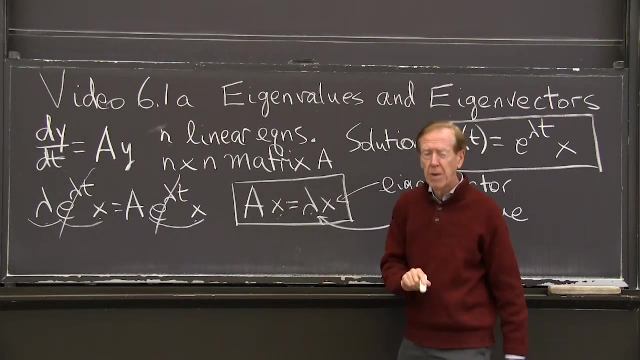 So I cancel e to the lambda t, OK, Because it's never 0.. And I have the big equation: Ax, the matrix times my eigenvector, is equal to lambda x, The number, the eigenvalue times the eigenvector. 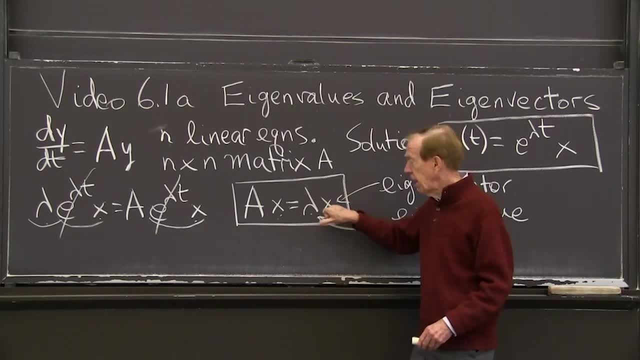 Not linear notice. Two unknowns here that are multiplied A number lambda times a: vector x. So what am I looking for? I'm looking for vectors x, The eigenvectors, So that multiplying by a, multiplying a times x. 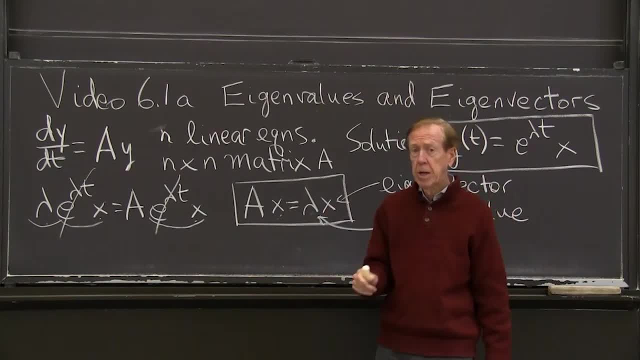 gives a number times x. It's in the same direction as x, just the length is changed. Well, if lambda was 1, I would have ax equal x. That's allowed. If lambda is 0, I would have ax equals 0.. 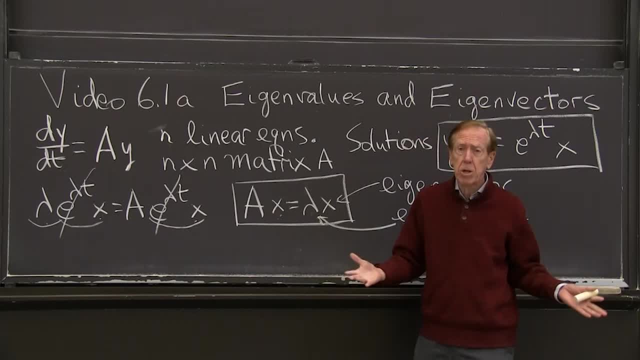 That's all right. I don't want x to be 0. That's useless. That's no help to know that 0 is a solution. So x should be not 0.. Lambda can be any number And it can be real. 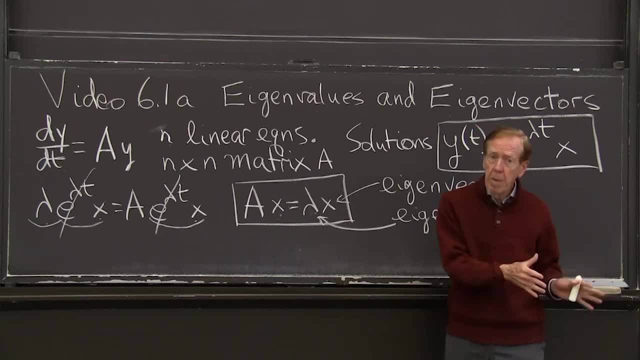 It could be complex number. as you will see, Even if the matrix is real, lambda could be complex. Anyway, ax equal lambda x. That's the big equation. It got a box around it, OK. So now I'm ready to do an example. 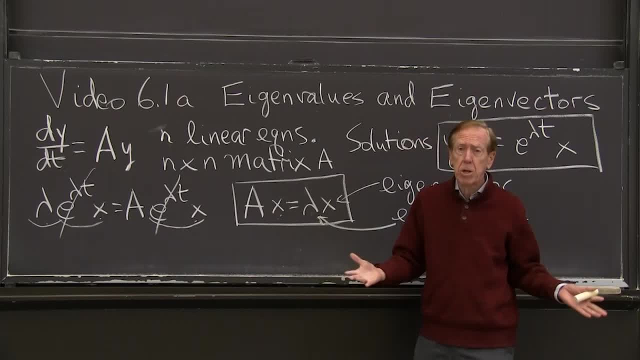 That's all right. I don't want x to be 0. That's useless. That's no help to know that 0 is a solution. So x should be not 0.. Lambda can be any number And it can be real. 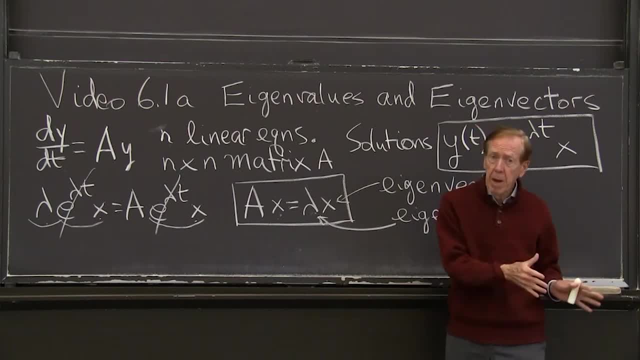 It could be complex number. as you will see, Even if the matrix is real, lambda could be complex. Anyway, ax equal lambda x. That's the big equation. It got a box around it, OK. So now I'm ready to do an example. 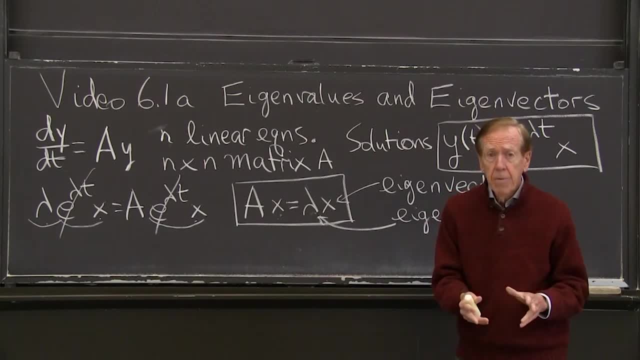 OK, And in this example, first of all, I'm going to spot the eigenvalues and eigenvectors without a system. Just go for it in the 2 by 2 case. OK, So I'll give a 2 by 2 matrix A We'll. 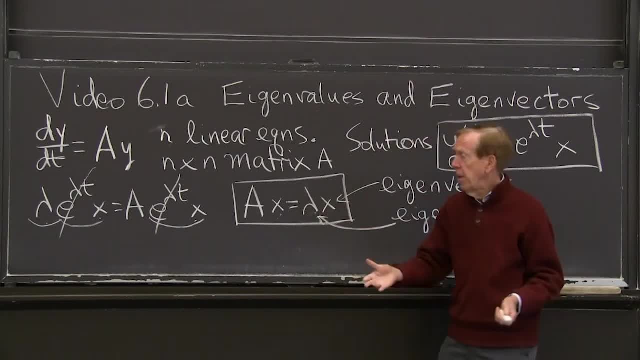 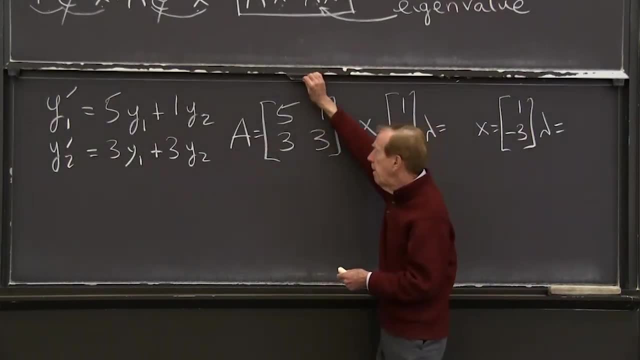 find the lambdas and the x's, And then we'll have the solution to the system of differential equations. Good, OK, There's the system. There's the first one. There's the first one, There's the first equation for y1.. 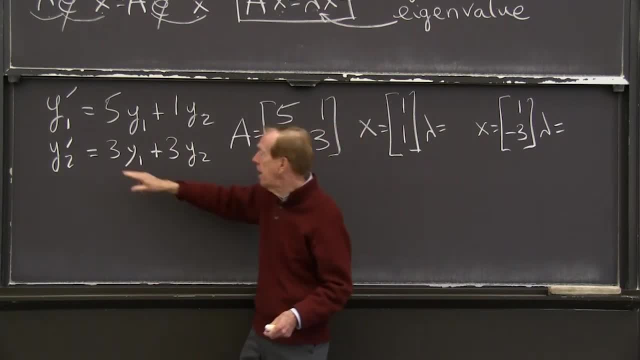 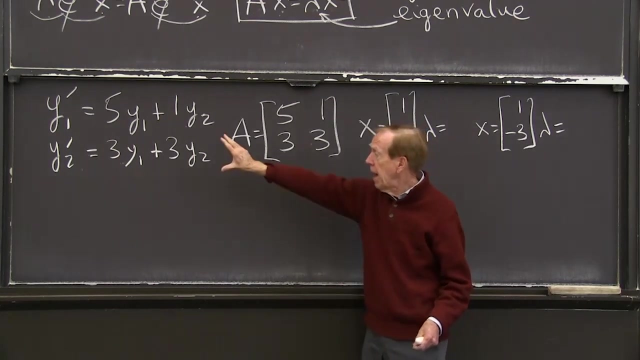 Prime, meaning derivative d by dt time derivative is a linear constant coefficient. Second one linear constant coefficients 3 and 3.. Those numbers 5, 1, 3, 3, go into the matrix. Then that problem is exactly y prime, the vector. 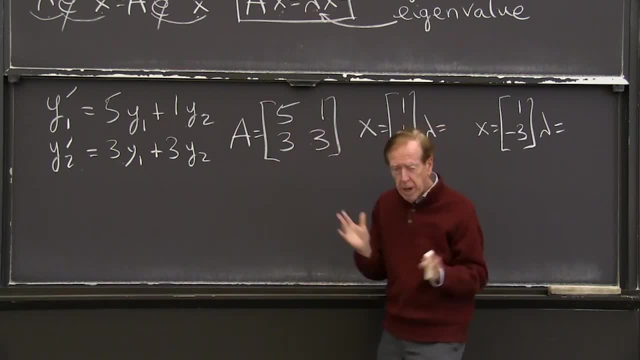 Derivative of the vector equal A times y. OK, That's my problem Now. eigenvalues and eigenvectors will solve it. OK, So I just look at that matrix Matrix question. What are the eigenvalues, What are the eigenvectors of that matrix? 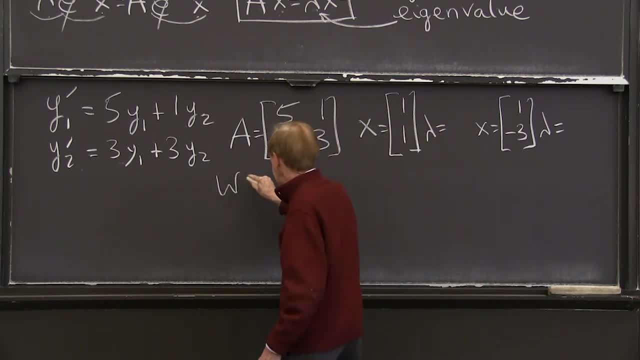 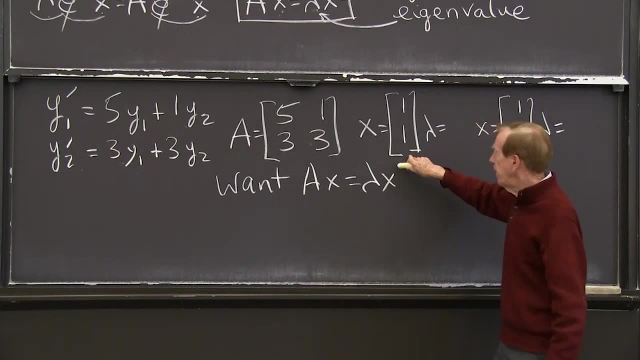 OK, And remember I want Ax equals lambda x. I've spotted the first eigenvector. Why? Why 1, 1.. We can just check: Does it work If I multiply A by that eigenvector 1, 1,? 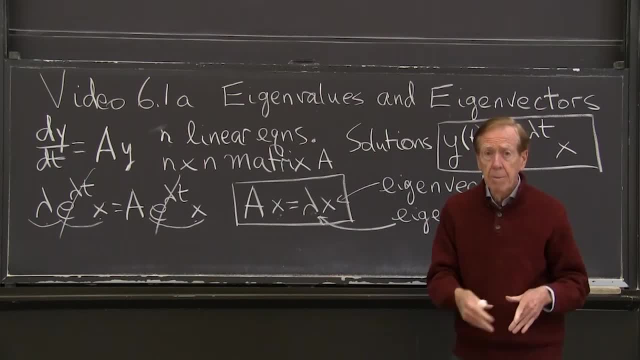 And in this example, first of all, I'm going to spot the eigenvalues and eigenvectors without a system. Just go for it in the 2 by 2 case. OK, So I'll give a 2 by 2 matrix A We'll. 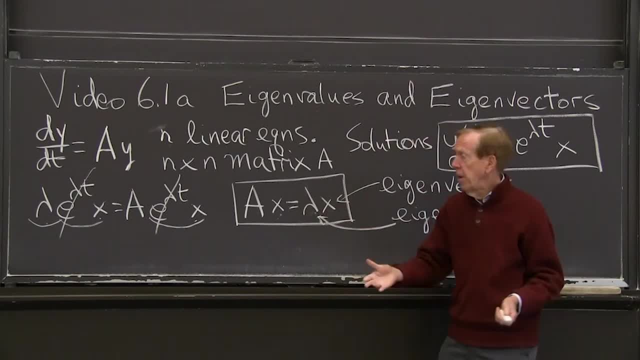 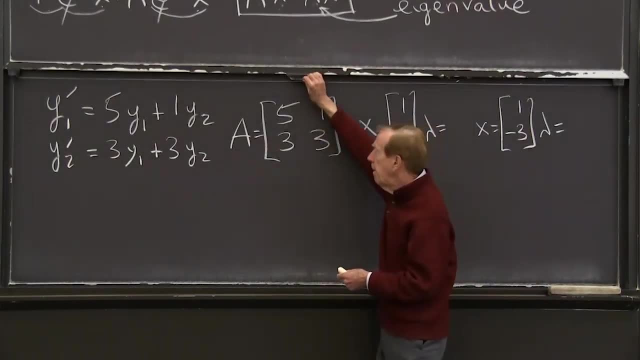 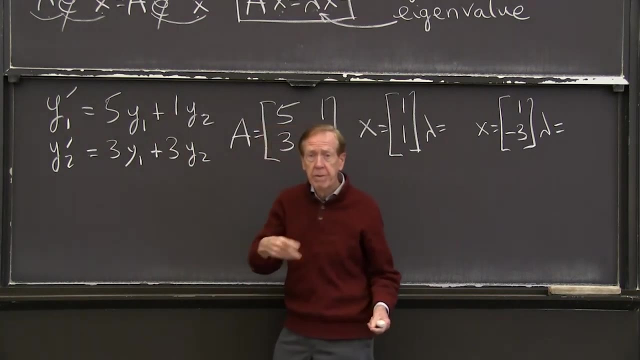 find the lambdas and the x's, And then we'll have the solution to the system of differential equations. Good, OK, There's the system, There's the function. There's the function, The first equation for y1 prime, meaning derivative d by dt. 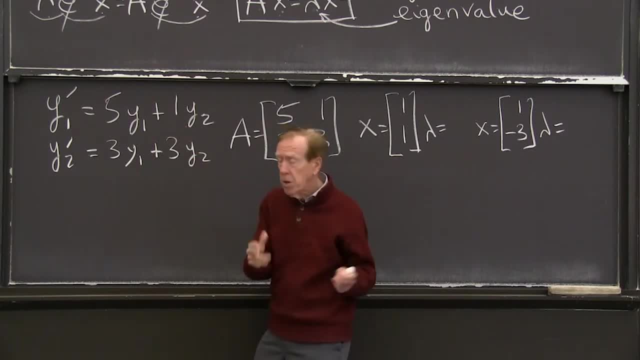 time derivative is linear constant coefficients. Second one: linear constant coefficients 3 and 3. Those numbers, 5, 1,, 3, 3 go into the matrix. Then that problem is exactly y prime the vector, derivative of the vector equal A times y. 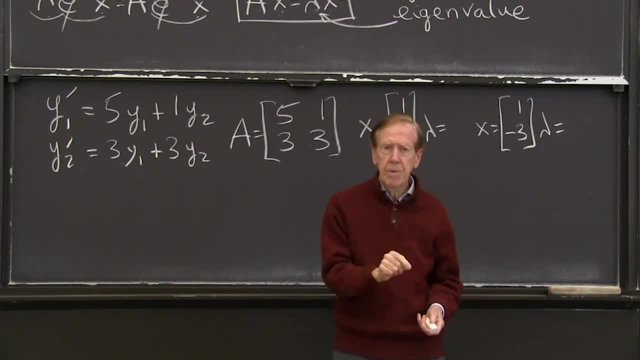 OK, That's my problem. Now, eigenvalues and eigenvectors will solve it. OK, So I just look at that matrix Matrix question: What are the eigenvalues, What are the eigenvectors of that matrix? OK, And remember I want Ax equals lambda x. 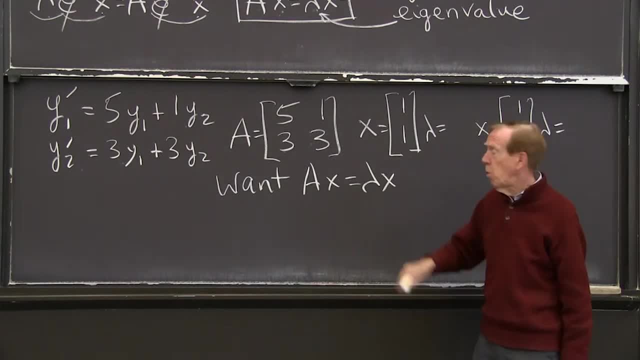 I've spotted the first eigenvector. Why 1, 1.. We can just check: Does it work If I multiply A by that eigenvector 1, 1, do you see what happens when I multiply by 1?? 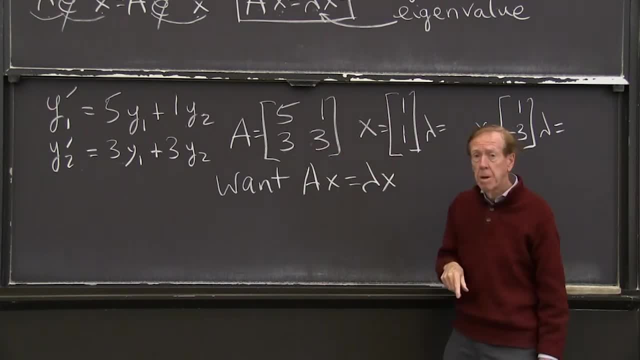 That gives me a 6.. That gives me a 6.. So A times that vector is 6, 6. And that is 6 times 1, 1.. So there you go, Found the first eigenvalue If I multiply A. 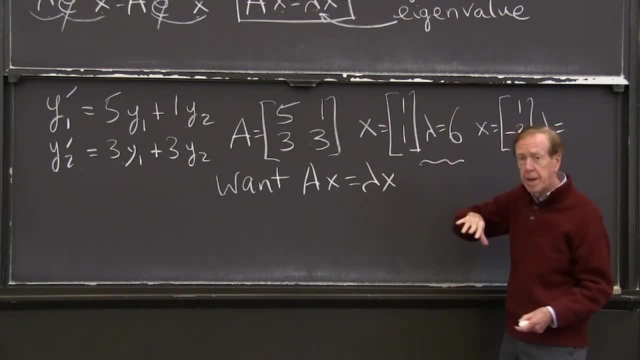 A by x, I get 6. by x, I get the vector 6, 6.. Now the second one. Again, I've worked in advance, produced this eigenvector And I think it's 1 minus 3.. 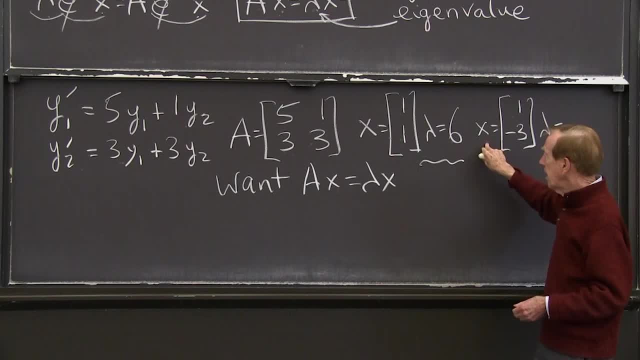 So let's multiply by A Try the second eigenvector. I should call this first one maybe x1 and lambda 1. And I should call this one x2 and lambda 2. And we can find out what lambda 2 is. 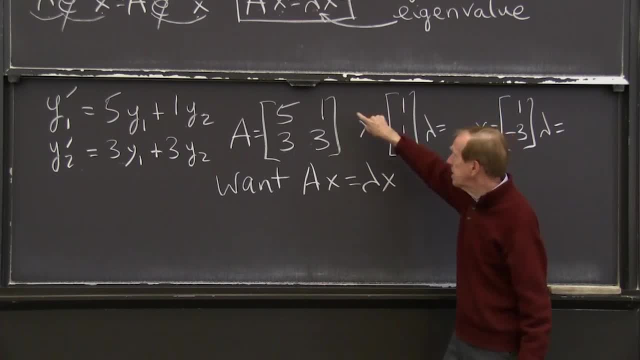 do you see what happens when I multiply by 1? That gives me a 6.. That gives me a 6.. So A times that vector is 6, 6. And that is 6 times 1, 1.. So there you go. 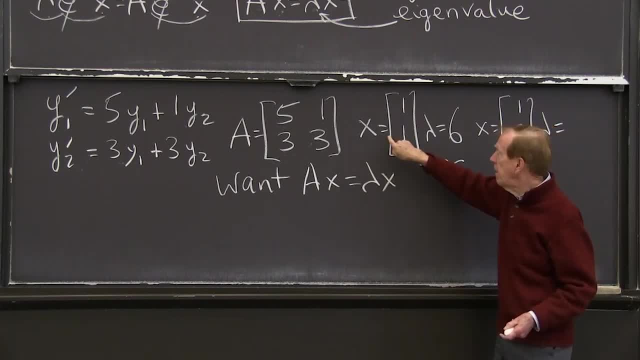 Found the first eigenvalue. If I multiply A, A by x, I get 6 by x, I get the vector 6, 6.. Now the second one. Again, I've worked in advance, produced this eigenvector. 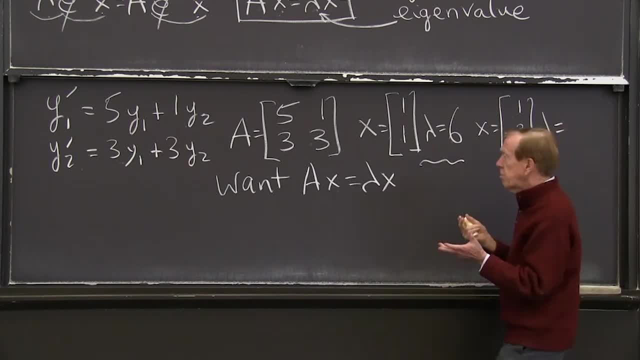 And I think it's 1 minus 3.. So let's multiply by A. Try the second eigenvector. I should call this first one maybe x1 and lambda 1.. And I should call this one x2 and lambda 2.. 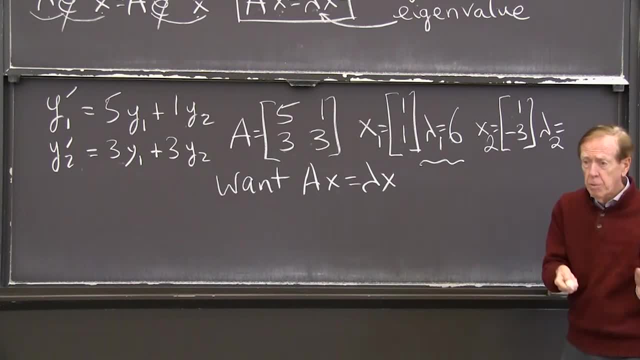 And we can find out what lambda 2 is, If I know. once I find the eigenvectors, of course, I just do A times x to recognize the lambda, the eigenvalue. So 5, 1 times this is 5 minus 3 is a 2.. 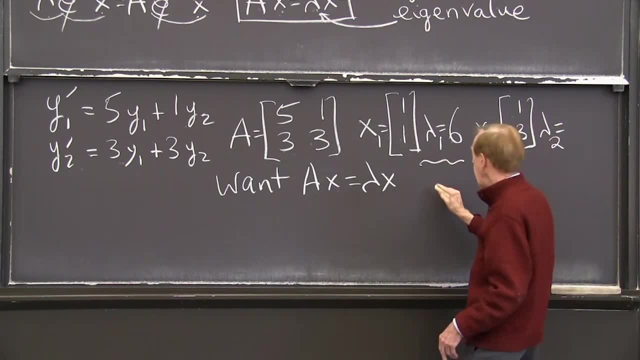 It's a 2.. So here I got a 2. And from 3, 3, it's 3 minus 9 is minus 6.. That's what I got. for Ax, There was the x. When I did the multiplication, Ax came out to be 2 minus 6.. 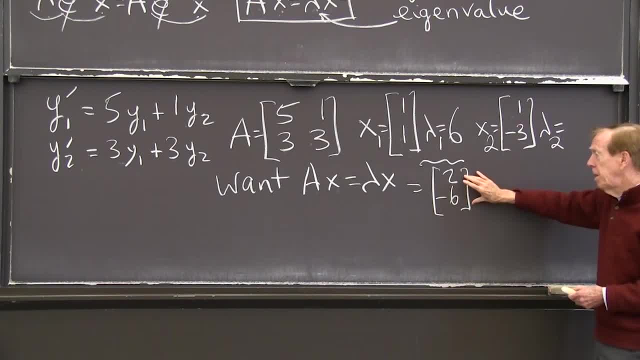 And good, That output is 2 times the input, The eigenvalue is 2.. Right, I'm looking for inputs, the eigenvector, so that the output is a number times that eigenvector And that number is lambda, the eigenvalue. 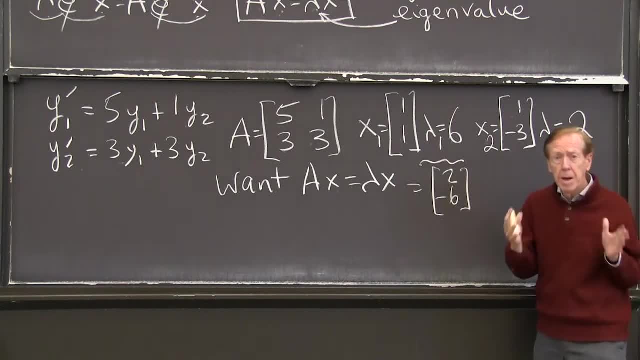 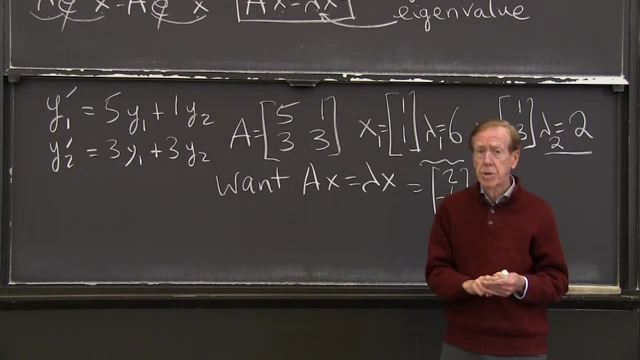 So I have now found the 2. And I expect 2. For a 2 by 2 matrix. you'll soon see why I expect 2 eigenvalues, And each eigenvalue should have an eigenvector. So here they are for this matrix. 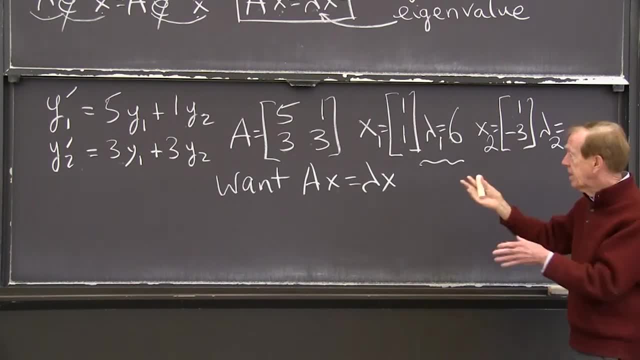 If I know. once I find the eigenvectors, of course I just do A times x to recognize the lambda, the eigenvalue. So 5, 1 times this is 5 minus 3 is a 2. It's a 2.. 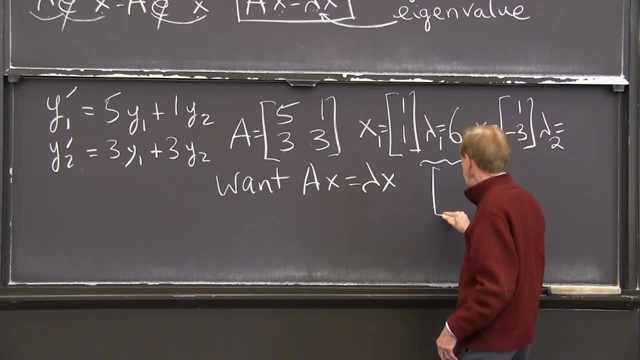 So here I got a 2. And from 3,, 3, it's 3 minus 9 is minus 6.. That's what I got. for Ax, There was the x. When I did the multiplication, Ax came out to be 2 minus 6.. 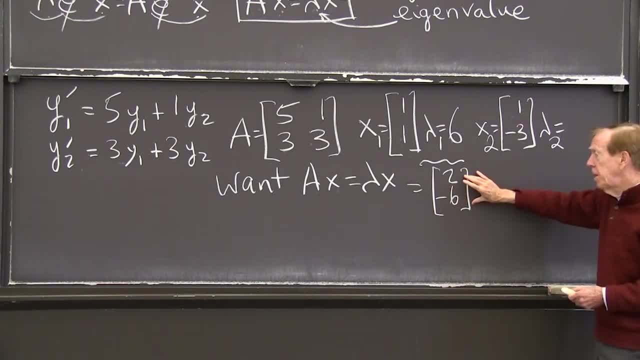 And good, That output is 2 times the input, The eigenvalue is 2.. Right, I'm looking for inputs, the eigenvector, so that the output is a number times that eigenvector And that number is lambda, the eigenvalue. 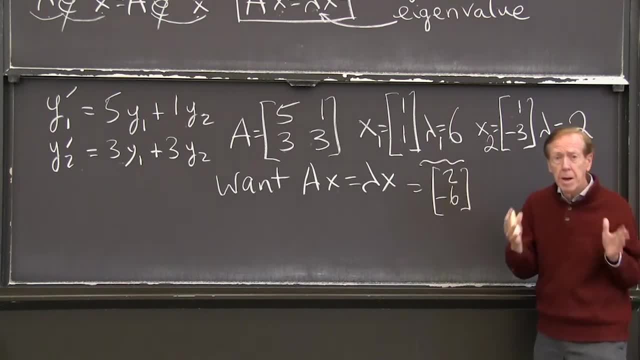 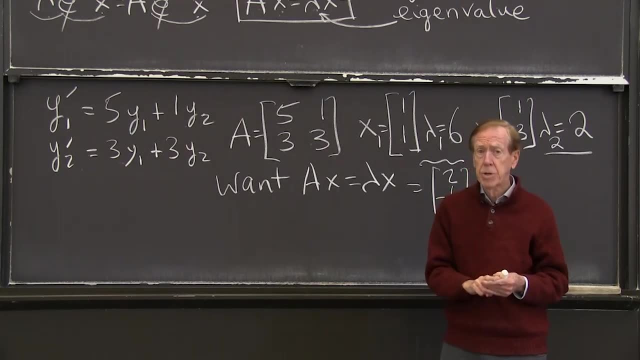 So I have now found the 2. And I expect 2. For a 2 by 2 matrix. you'll soon see why I expect 2 eigenvalues, And each eigenvalue should have an eigenvector. So here they are for this matrix. 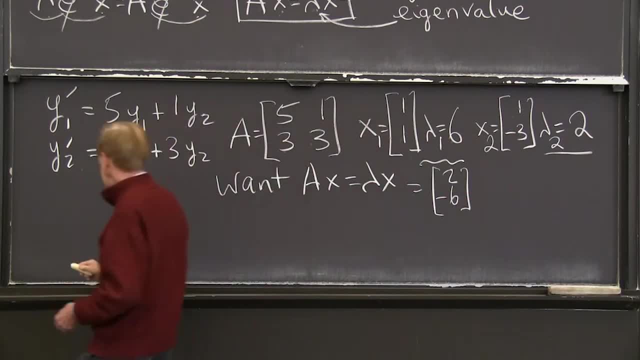 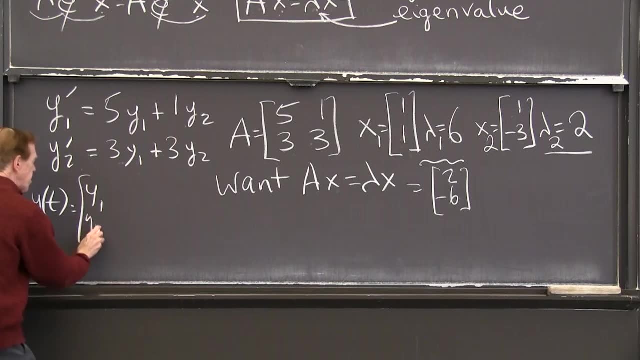 So I've got the answers now: y of t, Which stands for y1, and y2 of t. Those are OK. it's e to the lambda tx. Remember, that's the picture that we're looking for. So the first one is e to the 6t times x, which is 1, 1.. 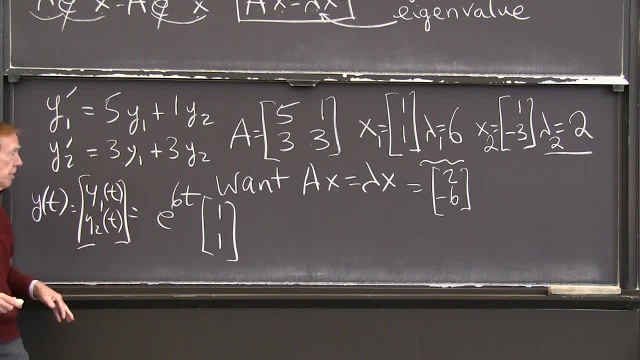 If I put that into the equation, it will solve the equation Also. I have another one: e to the lambda 2 was 2t. e to the lambda t times its eigenvector 1 minus 3.. That's a solution also. 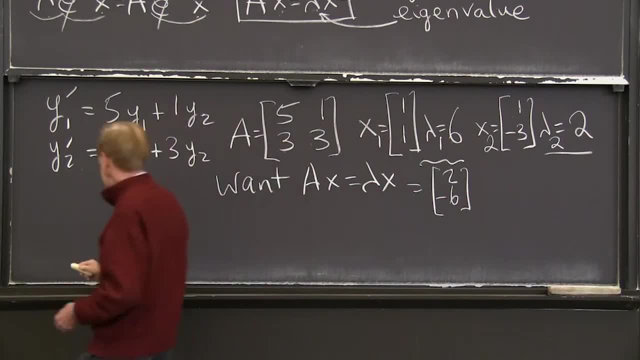 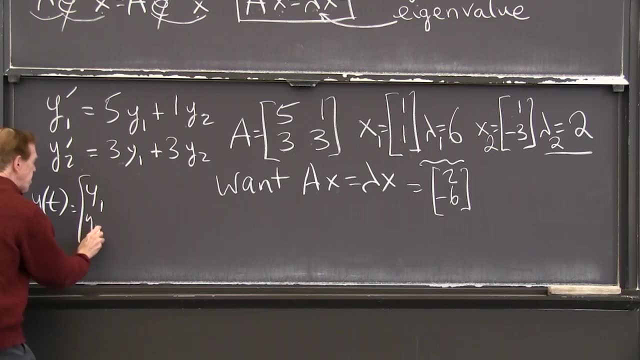 So I've got the answers now: y of t, Which stands for y1, and y2 of t. Those are OK. it's e to the lambda tx. Remember, that's the picture that we're looking for. So the first one is e to the 6t times x, which is 1, 1.. 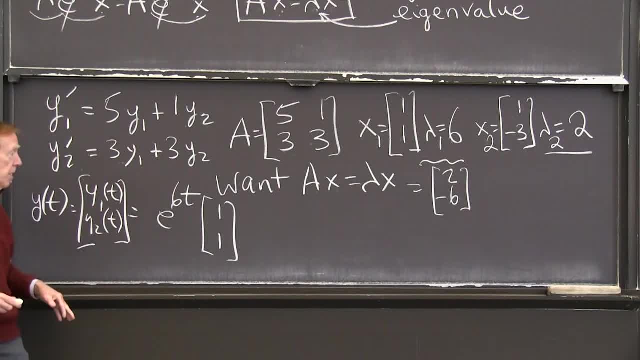 If I put that into the equation, it will solve the equation Also. I have another one: e to the lambda 2 was 2t. e to the lambda t times its eigenvector 1 minus 3.. That's a solution also. 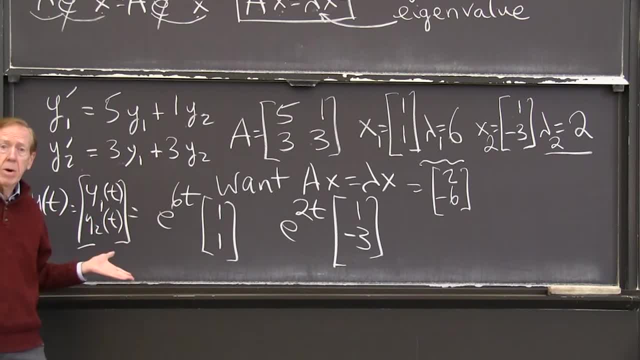 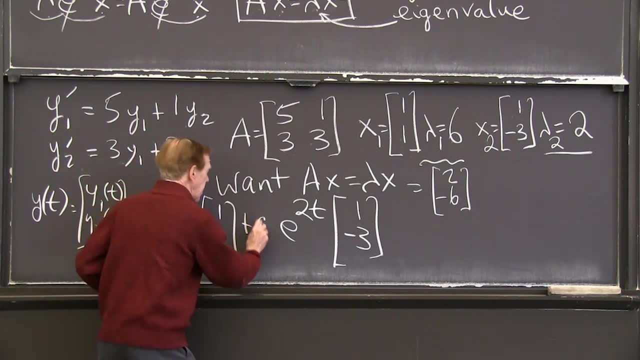 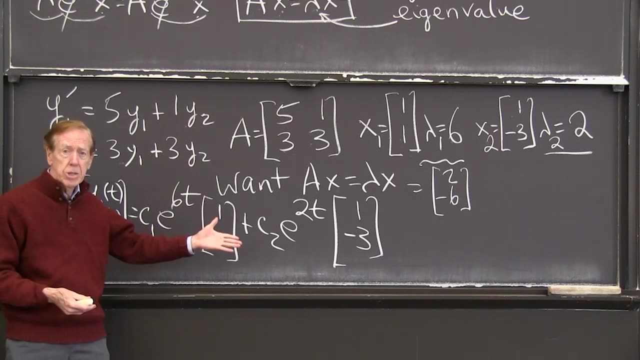 One solution, another solution. And what do I do with linear equations? I take combinations: any number c1 of that plus any number c2 of that, That is still a solution. That's superposition, adding solutions to linear equations. These are null equations. 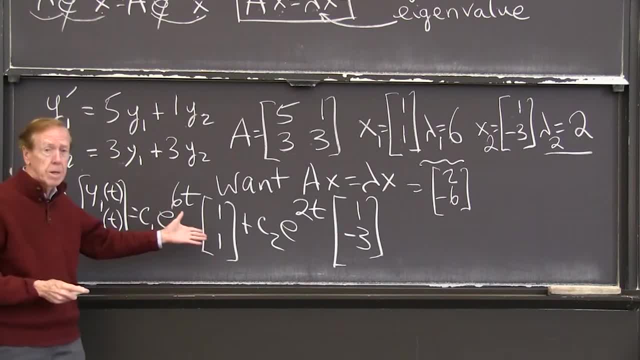 There's no force term in these equations. I'm not dealing with a force term. I'm looking for the null solutions, the solutions of the equations themselves. And there I have two solutions, two coefficients to choose. How do I choose them? 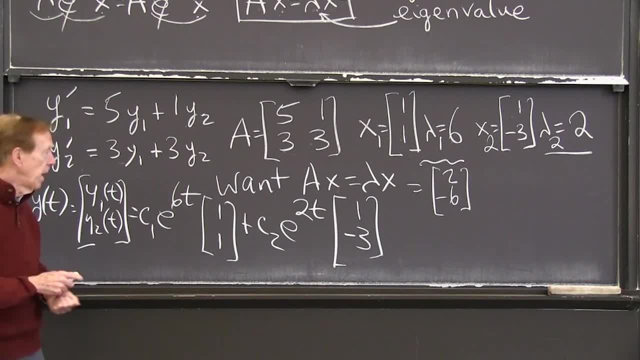 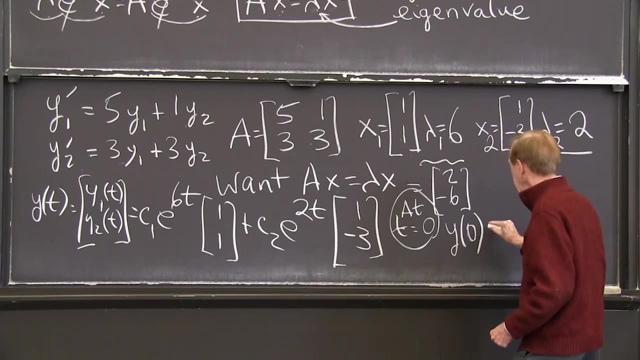 Of course I match the initial condition. So, at t equals 0,, I would have y of 0. That's my given initial condition, my y1 and y2.. So I'm setting t equals 0. So that's 1, of course. 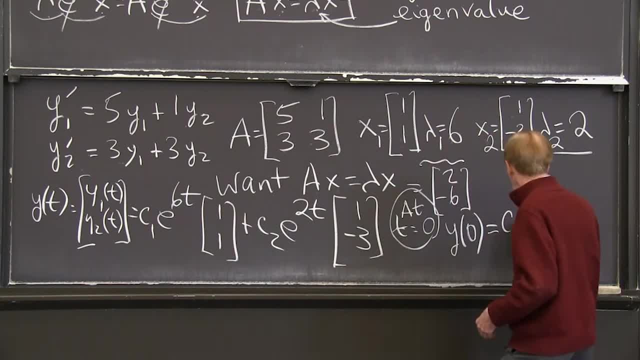 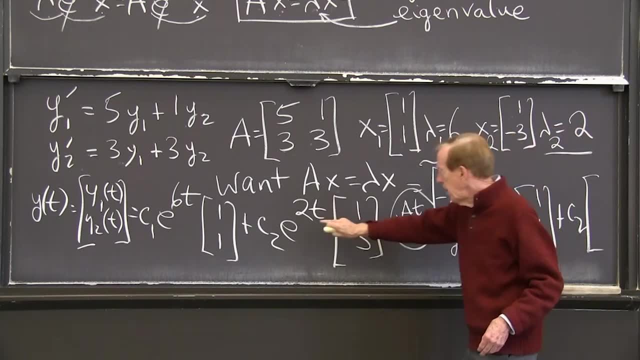 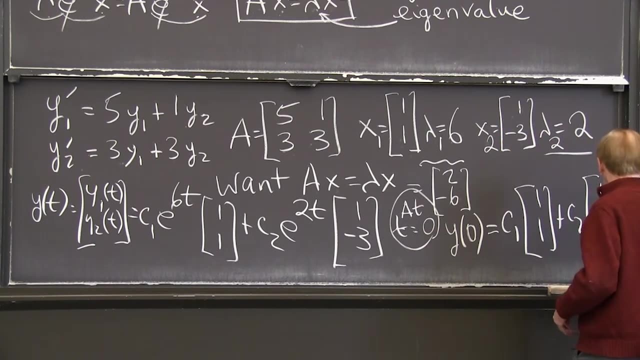 When t is 0,, that's 1.. So I just have c1 times 1, 1.. And c2 times that's 1 again at t equals 0, times 1 minus 3.. That's what determines c1 and c2.. 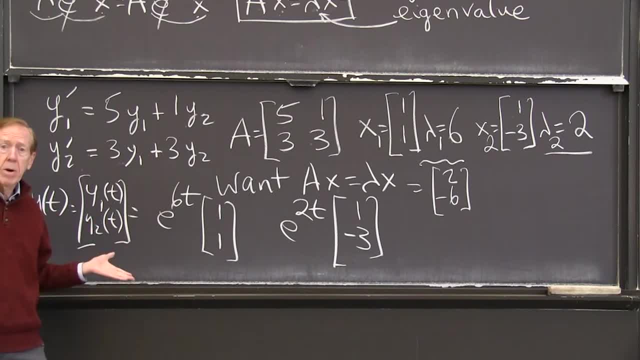 One solution, another solution. And what do I do with linear equations? I take combinations: any number c1 of that plus any number c2 of that, That is still a solution. That's superposition, adding solutions to linear equations. These are null equations. 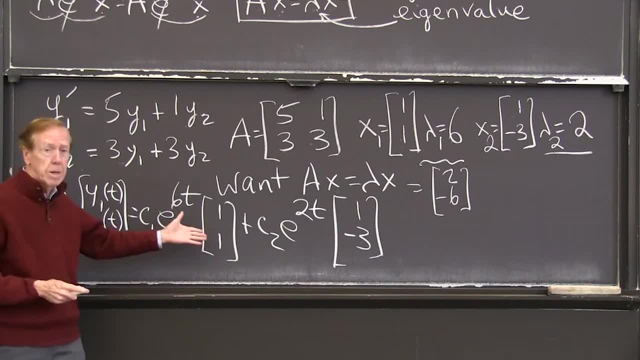 There's no force term in these equations. I'm not dealing with a force term. I'm looking for the null solutions, the solutions of the equations themselves. And there I have two solutions, two coefficients to choose. How do I choose them? 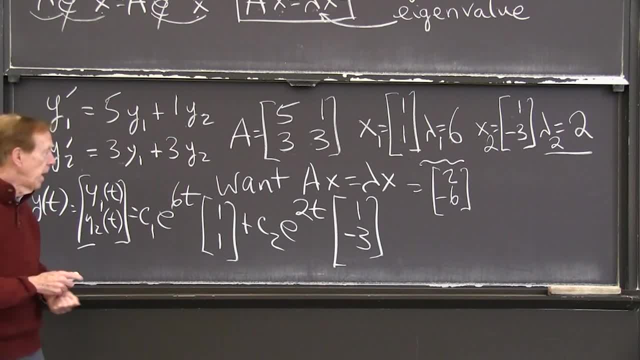 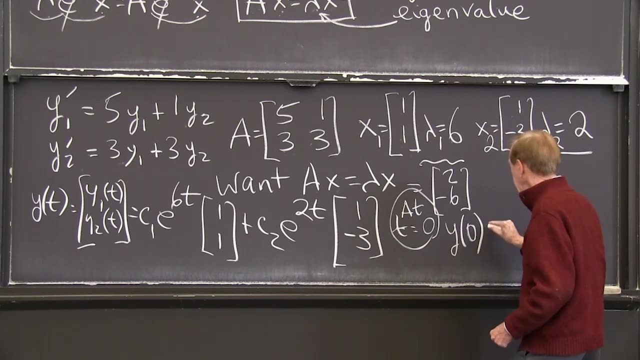 Of course I match the initial condition. So, at t equals 0,, I would have y of 0. That's my given initial condition, my y1 and y2.. So I'm setting t equals 0. So that's 1, of course. 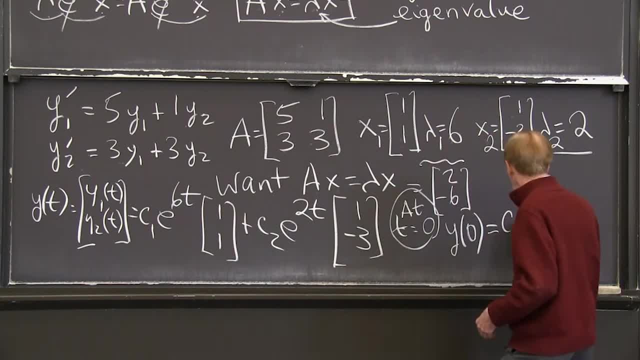 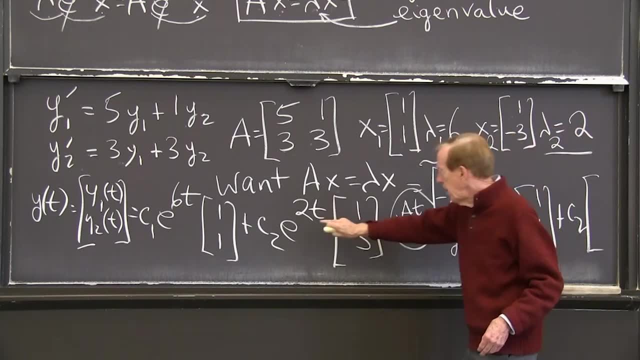 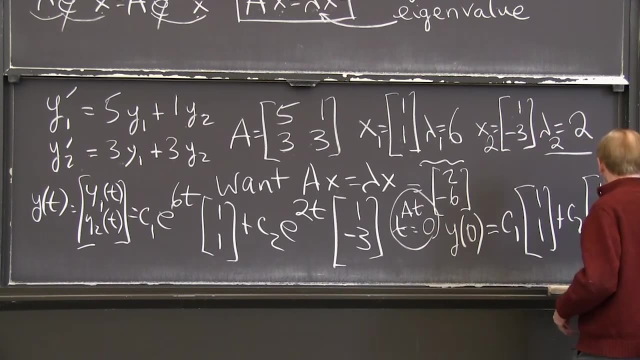 When t is 0,, that's 1.. So I just have c1 times 1, 1.. And c2 times that's 1 again at t equals 0, times 1 minus 3.. That's what determines c1 and c2.. 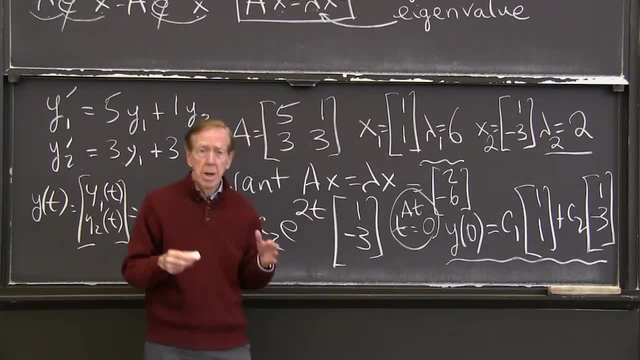 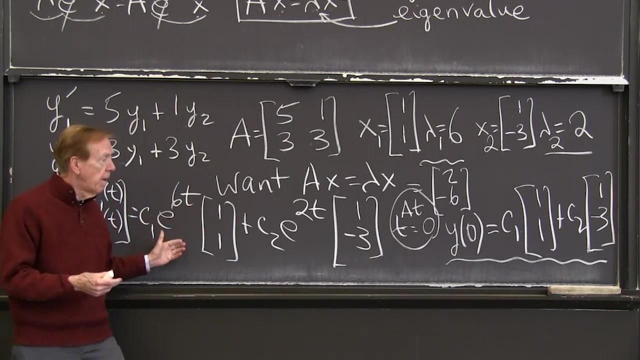 c1 and c2 come from the initial conditions, just the way they always did. So I'm solving two first order linear constant coefficient equations- homogeneous, meaning no force term, And so I get a null solution with constants to choose, And, as always, those constants come from matching. 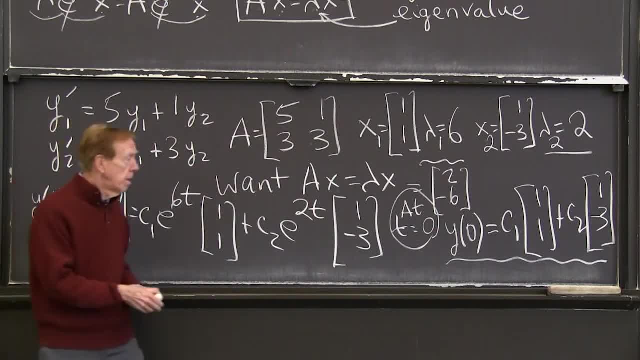 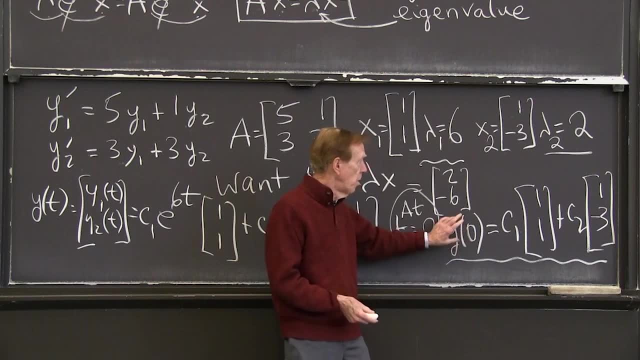 the initial conditions. So the initial condition here is a vector. So if, for example, y of 0 was 2 minus 2, then I would want one of those and one of those. OK, I've used eigenvalues and eigenvectors. 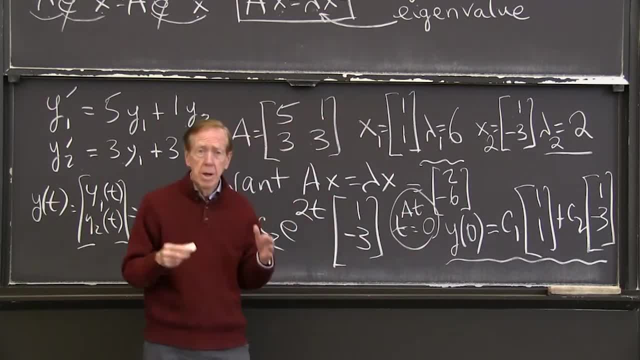 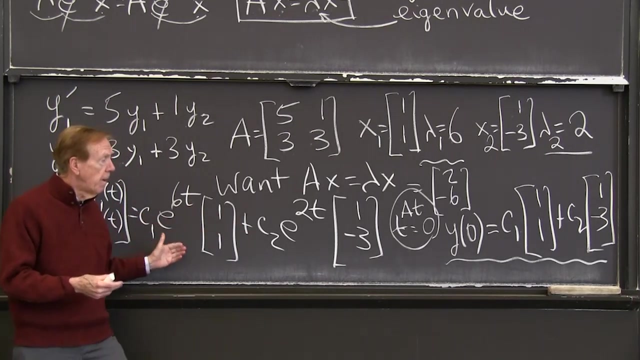 c1 and c2 come from the initial conditions, just the way they always did. So I'm solving two first order linear constant coefficient equations- homogeneous, meaning no force term, And so I get a null solution with constants to choose, And, as always, those constants come from matching. 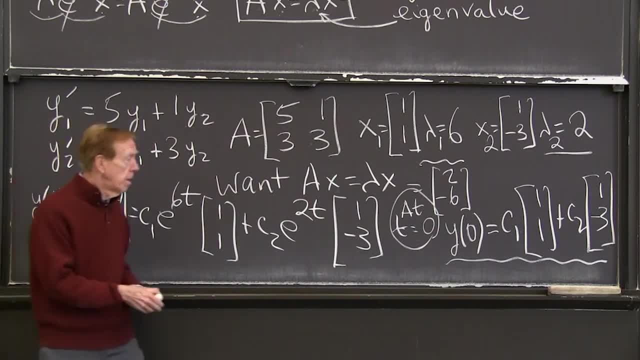 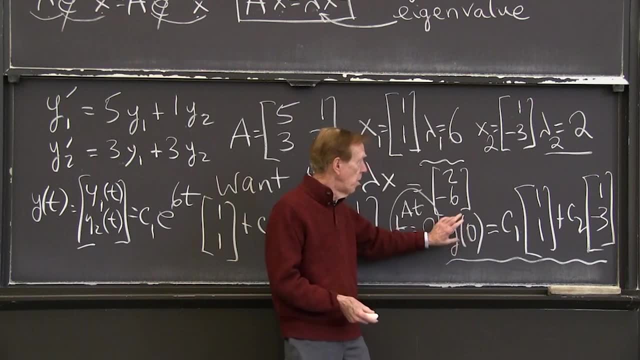 the initial conditions. So the initial condition here is a vector. So if, for example, y of 0 was 2 minus 2, then I would want one of those and one of those. OK, I've used eigenvalues and eigenvectors. 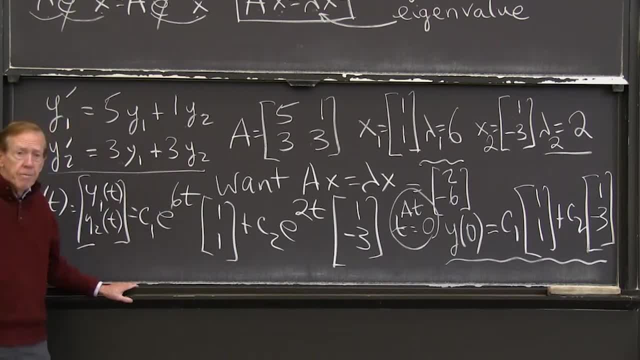 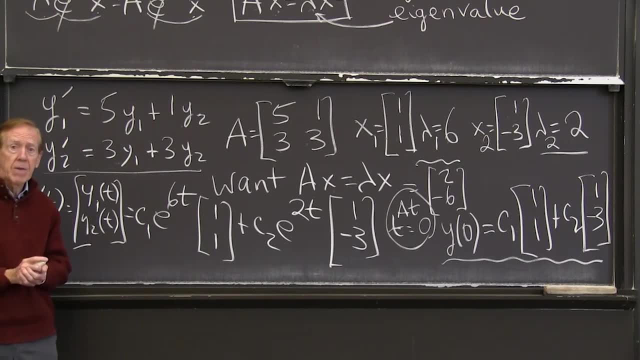 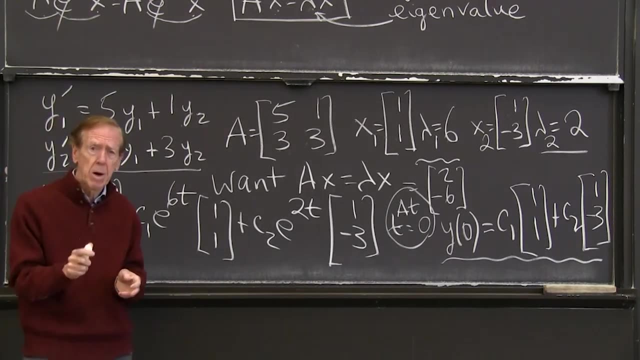 to solve a linear system, Their first and primary purpose. OK, But how do I find those eigenvalues and eigenvectors? What about other properties? What's going on with eigenvalues and eigenvectors? May I begin on this? Just a couple more minutes about eigenvalues and eigenvectors. 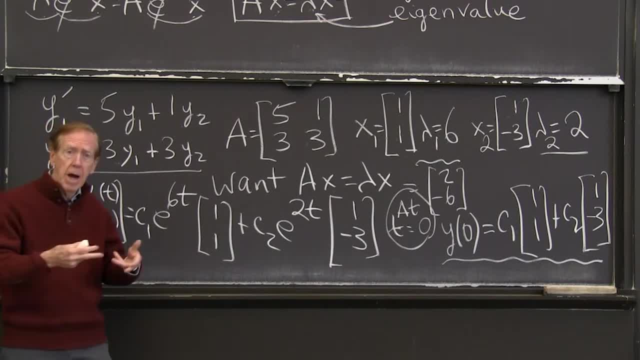 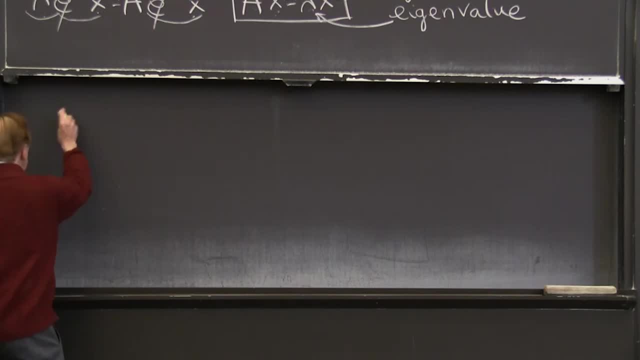 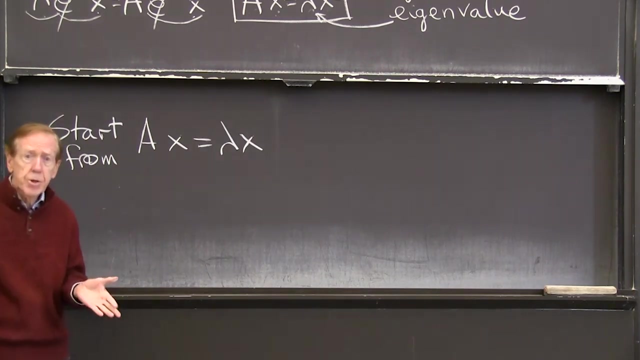 Basic facts And then I'll come next time, next video, of how to find them. OK, Basic facts, Basic facts. So start from: Ax equals lambda x. Let's suppose we found those. Could you tell me the eigenvalues and eigenvectors of a squared? 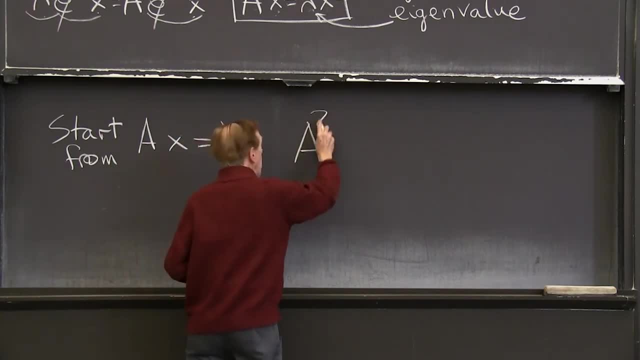 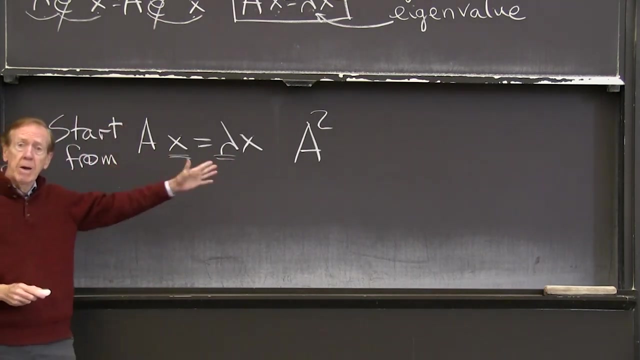 This is a. I would like to know what the eigenvalues and eigenvectors of a squared are. Are they connected with these? So I found the suppose I know the x and I know the lambda. What about for a? What about for a squared? 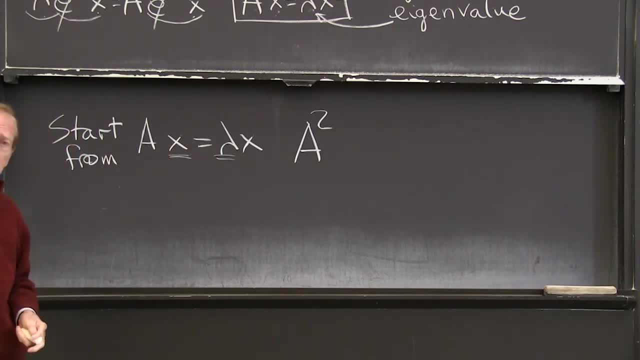 Well, the good thing is that the eigenvectors are the same for a squared. So let me show you. I say that: same x, so this is the same x, same vector, same eigenvector. The eigenvalue would be different, of course. 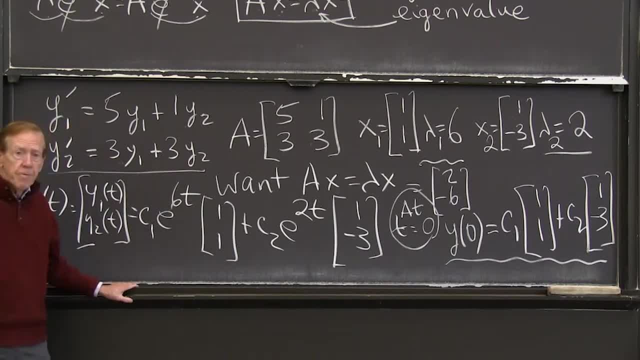 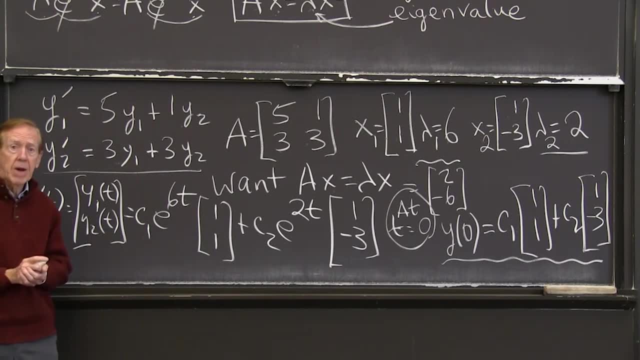 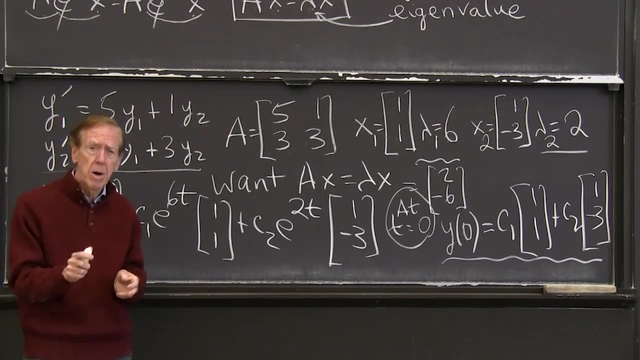 to solve a linear system. their first and primary purpose? OK, But how do I find those eigenvalues and eigenvectors? What about other properties? What's going on with eigenvalues and eigenvectors? May I begin on this. Just a couple more minutes about eigenvalues and eigenvectors. 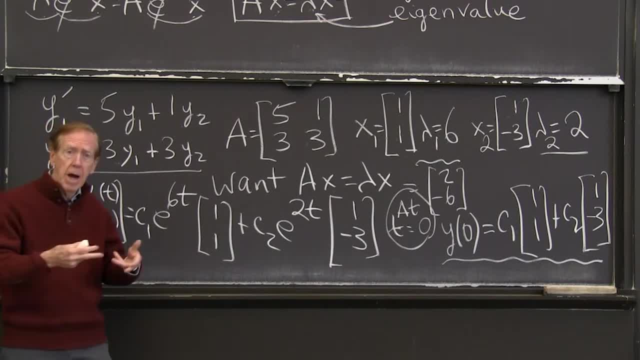 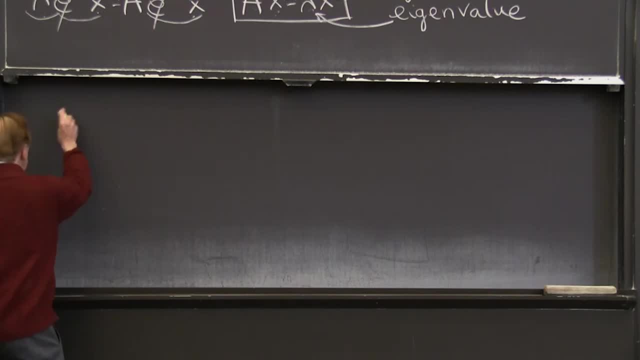 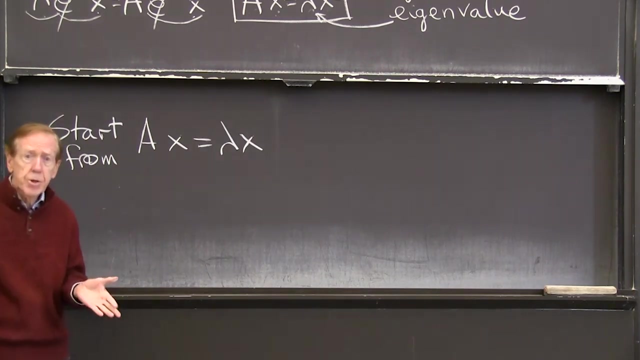 Basic facts And then I'll come next time, next video, of how to find them. OK, Basic facts, Basic facts. So start from: Ax equals lambda x. Let's suppose we found those. Could you tell me the eigenvalues and eigenvectors of a squared? 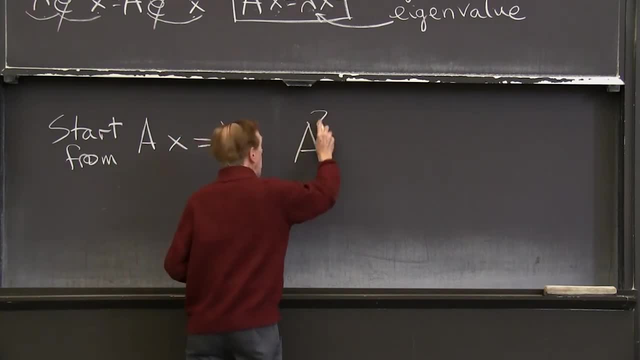 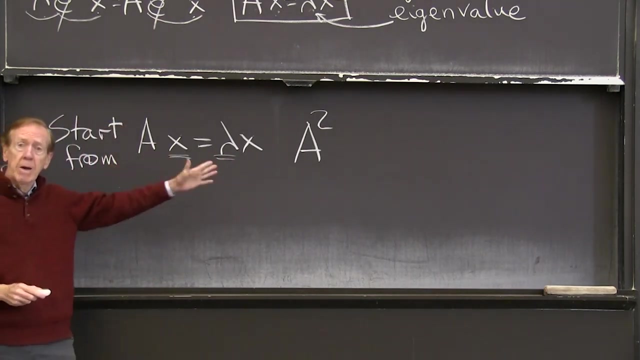 This is a. I would like to know what the eigenvalues and eigenvectors of a squared are. Are they connected with these? So I found the suppose I know the x and I know the lambda. What about for a? What about for a squared? 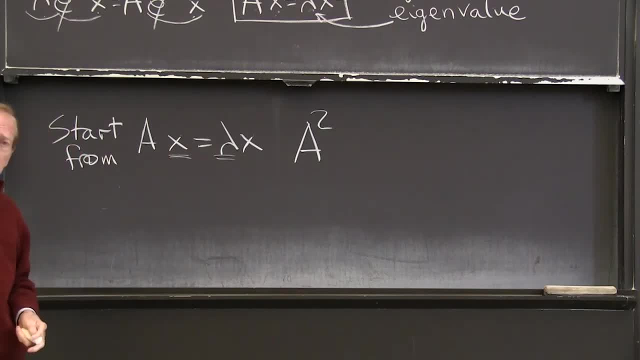 Well, the good thing is that the eigenvectors are the same for a squared. So let me show you. I say that: same x, so this is the same x, same vector, same eigenvector. The eigenvalue would be different, of course. 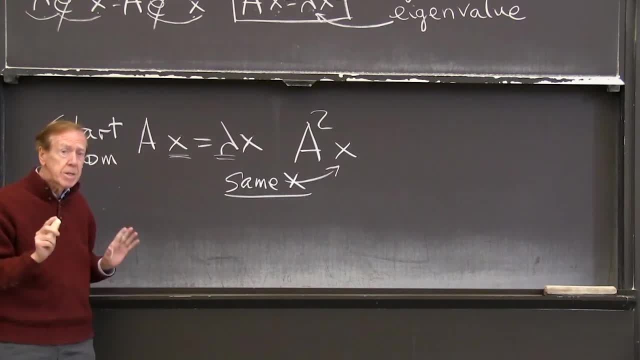 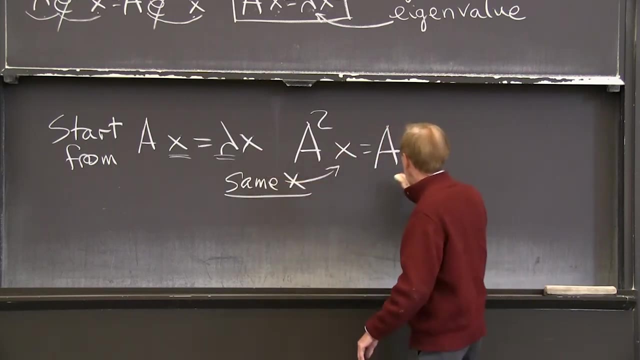 for a squared. But the eigenvector is the same. OK, And let's see what happens for a squared. So that's a times Ax, right, One, a times another Ax, but Ax is lambda x You good with that. 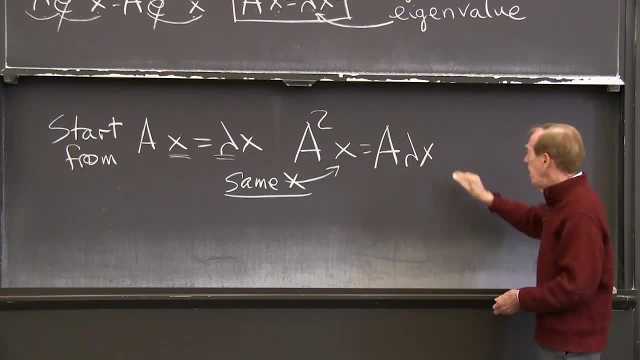 That's just a times Ax, so that's OK. Now lambda's a number. I'd like to bring it out front where I can see it, So I didn't do anything there. This number, lambda, was multiplying everything, so put it in front. 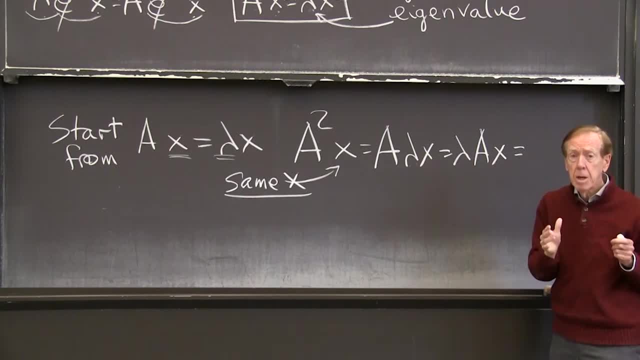 Now Ax, I have again the Ax. That's again the lambda x. because I'm looking at this: same x, same x, So I get the same lambda. so that's a lambda x, Another lambda. I have lambda squared x. 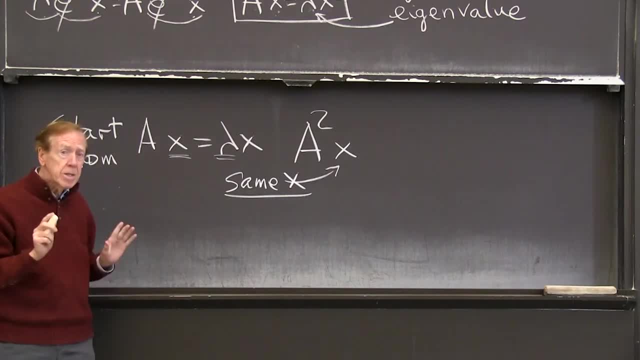 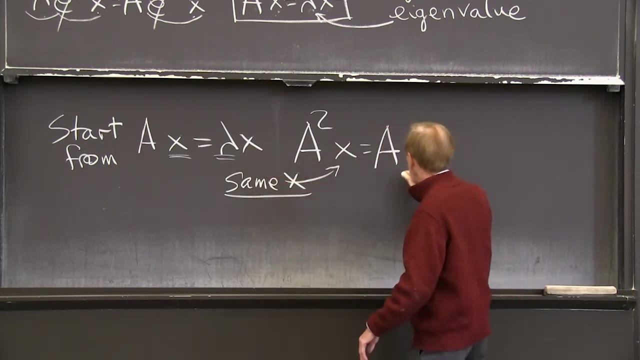 for a squared, But the eigenvector is the same. OK, And let's see what happens for a squared. So that's a squared A times Ax, right, One, a another Ax, But Ax is lambda x. Are you good with that? 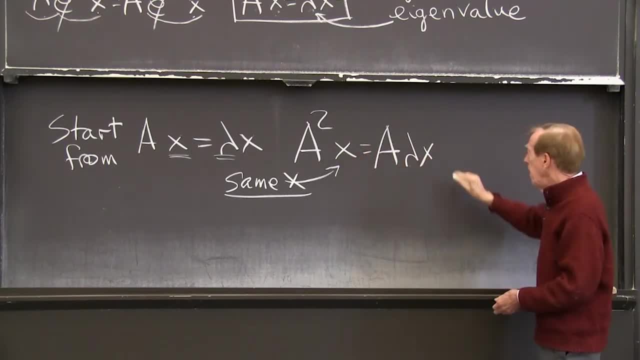 That's just a times Ax, so that's OK. Now lambda's a number. I'd like to bring it out front where I can see it, So I didn't do anything there. This number, lambda, was multiplying everything, so put it in front. 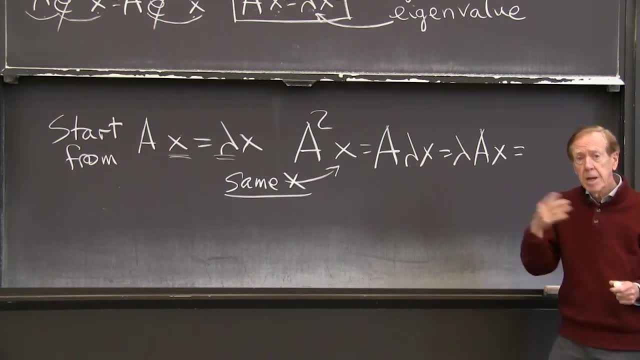 Now Ax, I have again the Ax. That's again the lambda x. because I'm looking at this: same x, same x, So I get the same lambda. So that's a lambda x, another lambda. I have lambda squared x. 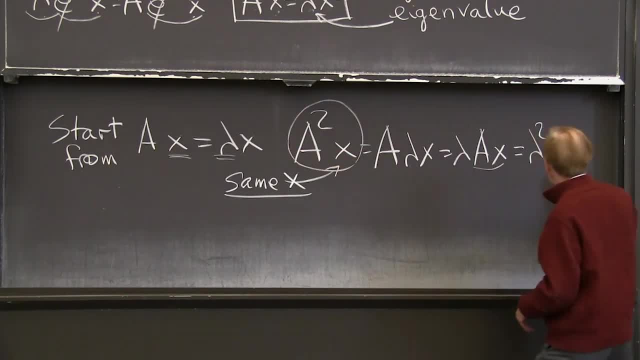 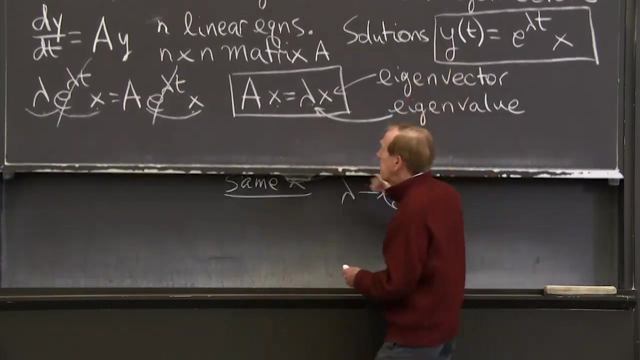 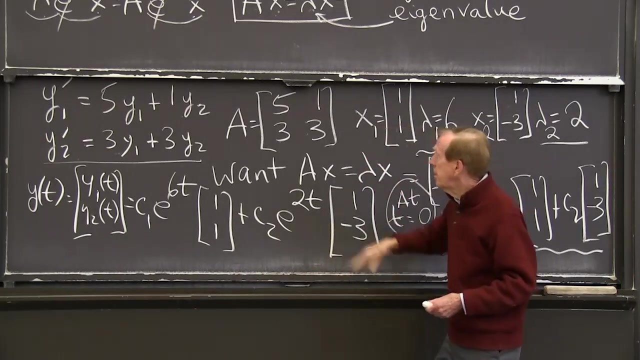 That's what I wanted. A squared x is lambda squared x. Conclusion: The eigenvectors stay. the same Lambda goes to lambda squared, The eigenvalues are squared. So if I had my example again, let me find that matrix. Suppose I had that same matrix and I 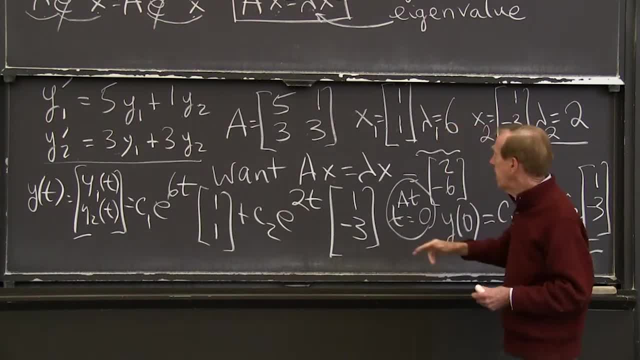 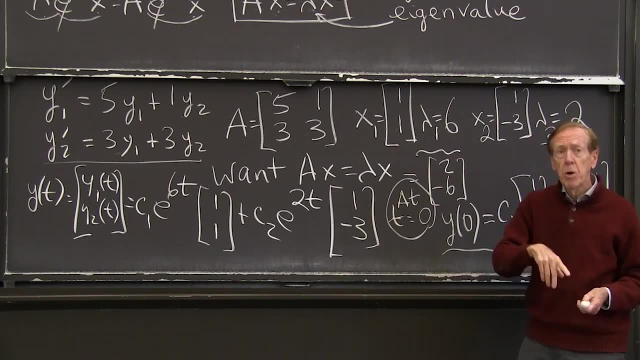 was interested in a squared, Then the eigenvalues would be 36 and 4, the squares. Suppose I'm looking at the n-th power of a matrix. You may say: why look at the n-th power? But there are many examples to look. 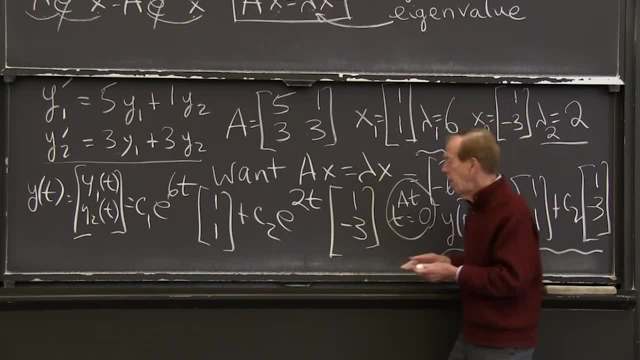 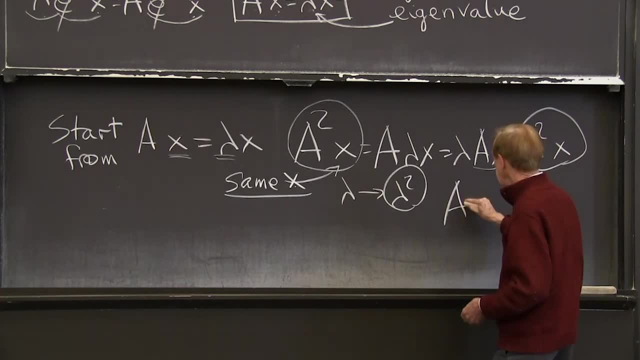 at the n-th power of a matrix, the thousandth power. So let's just write down the conclusion: same reasoning: A to the n-th x is lambda, It's the same x, And every time I multiply by A, I multiply. 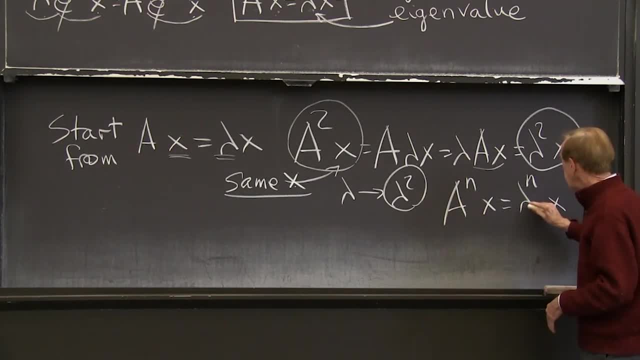 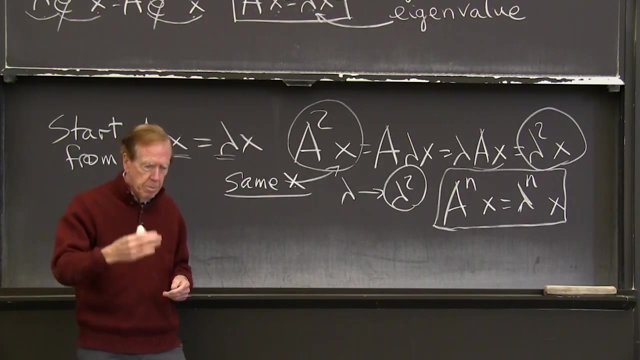 I multiply by a lambda, So I get lambda n times. So there's the handy rule That really tells us something about what eigenvalues are good for. Eigenvalues are good for things that move in time: differential equations. That is really moving in time. 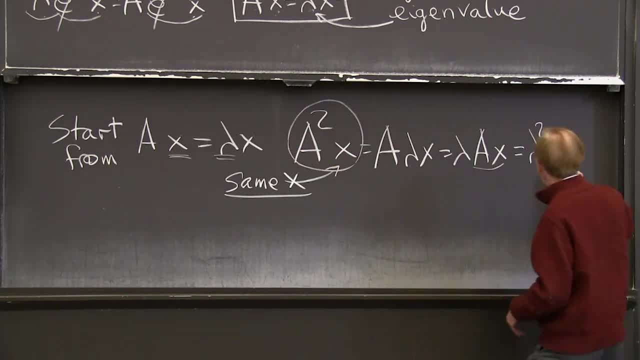 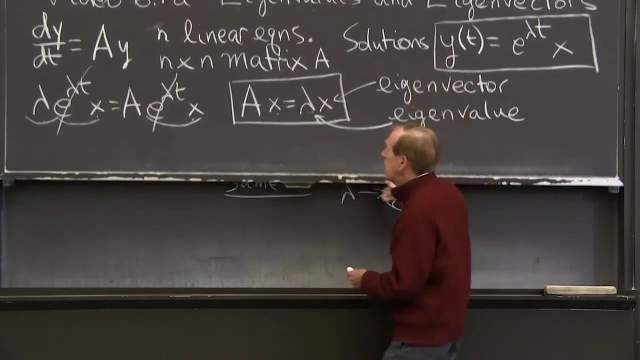 That's what I wanted. a squared x is lambda, squared x. Conclusion: The eigenvectors stay the same. Lambda goes to lambda, It goes to lambda squared, The eigenvalues are squared. So if I had my example again, let me find that matrix. 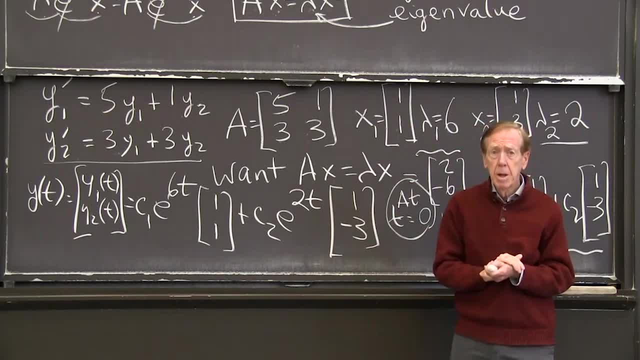 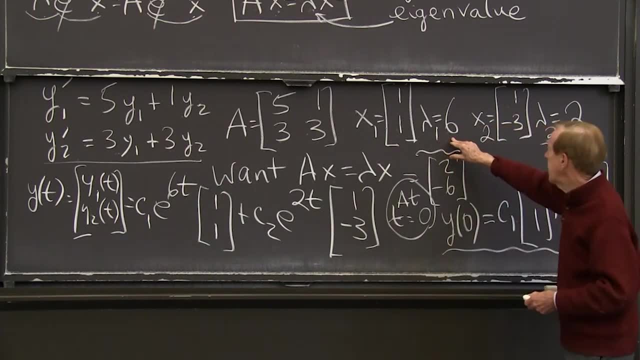 Suppose I had that same matrix and I was interested in a squared, Then the eigenvalues would be 36 and 4. They're squares. Suppose I'm looking at the nth power of a matrix, You may say why look at the nth power? 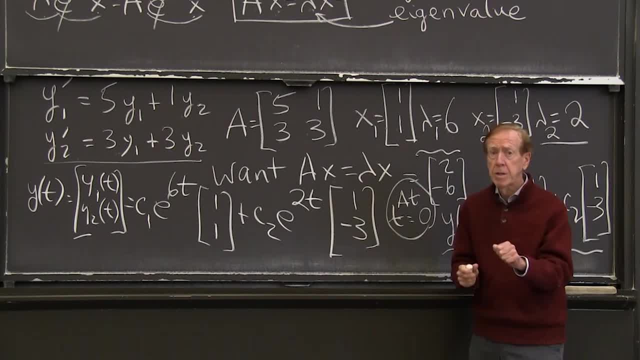 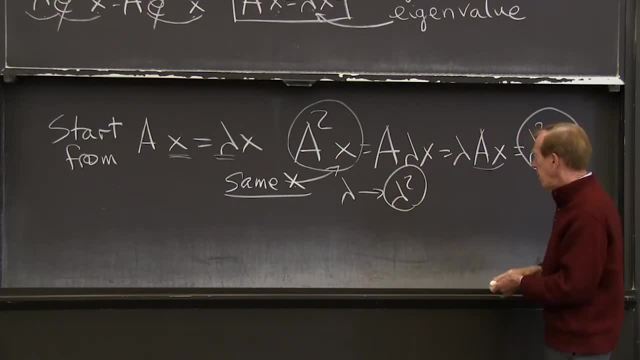 But there are many examples to look at the nth power of a matrix, the thousandth power. So let's just write down the conclusion: same reasoning: a to the nth x is lambda. It's the same x, And every time I multiply by a. 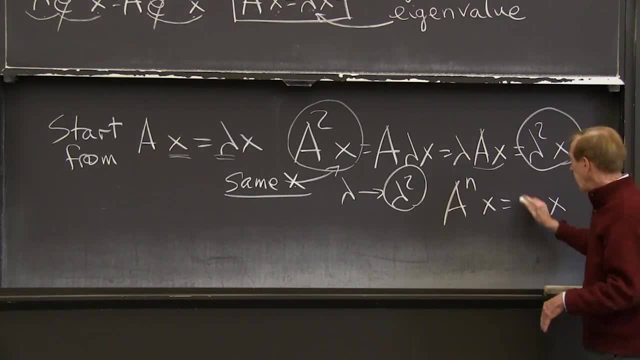 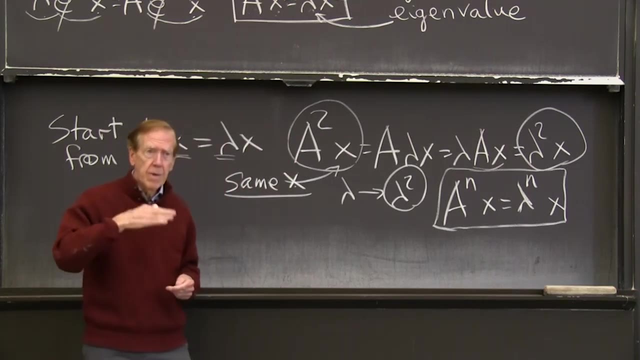 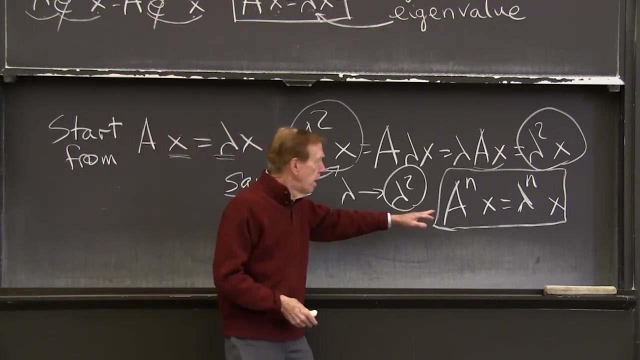 I multiply by a lambda, So I get lambda n times. So there's the handy rule That really tells us something about what eigenvalues are good for. Eigenvalues are good for things that move in time: Differential equations. That is really moving in time. 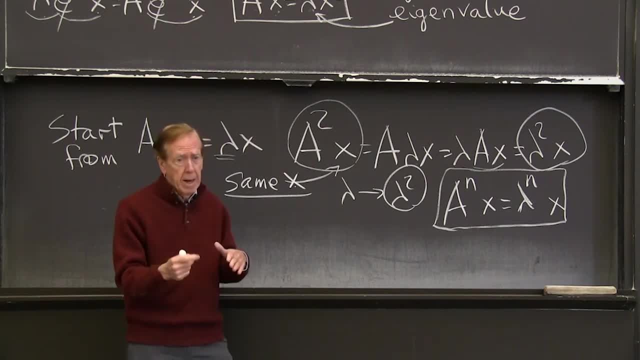 n equal 1 is the first First time, or n equals 0 is the start. Take one step to n equal 1.. Take another step to n equal 2.. Keep going Every time step brings a multiplication by lambda. So that is a very useful rule. 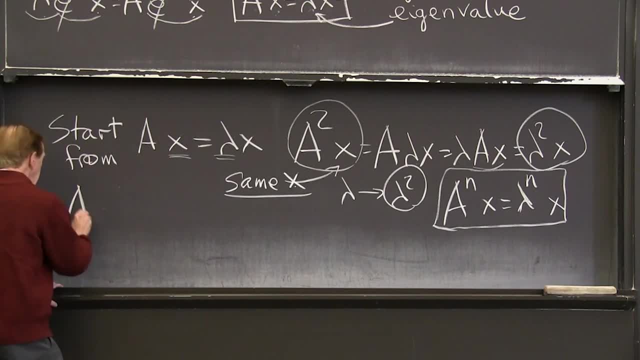 Another handy rule is: what about a plus the identity? Suppose I add the identity matrix. OK, I add the identity matrix to my original matrix. What happens to the eigenvalues? What happens to the eigenvectors? Basic question. Or I could multiply a constant times the identity. 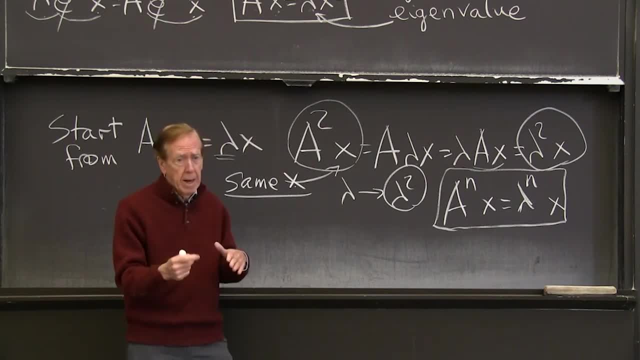 n equal 1 is the first time, Or n equals 0.. 0 is the start. Take one step to n equal 1.. Take another step to n equal 2.. Keep going Every time step brings a multiplication by lambda. 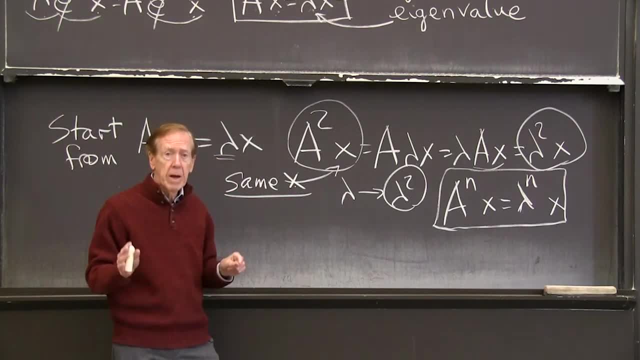 So that is a very useful rule. Another handy rule is: what about A plus the identity? Suppose I add the identity matrix To my original matrix. What happens to the eigenvalues? What happens to the eigenvectors? Basic question. 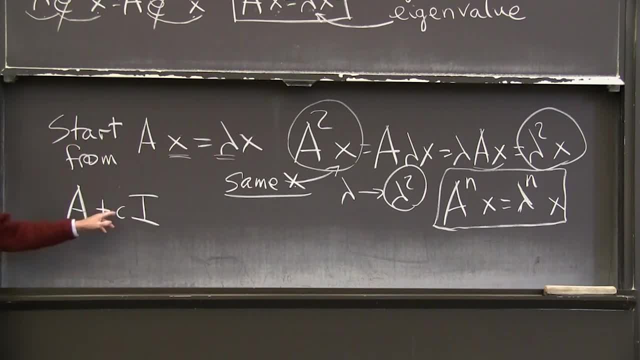 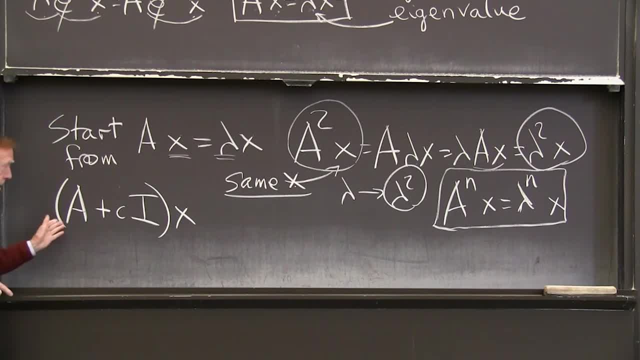 Same x, Same x. I show that by figuring out what I have here. This is Ax, which is lambda x, And this is C times the identity times x. The identity doesn't do anything, so that's just Cx. So what do I have now? 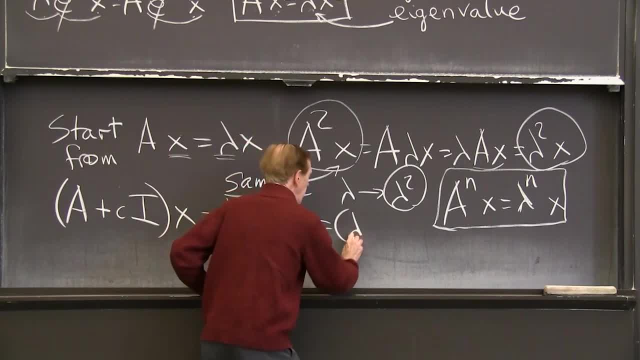 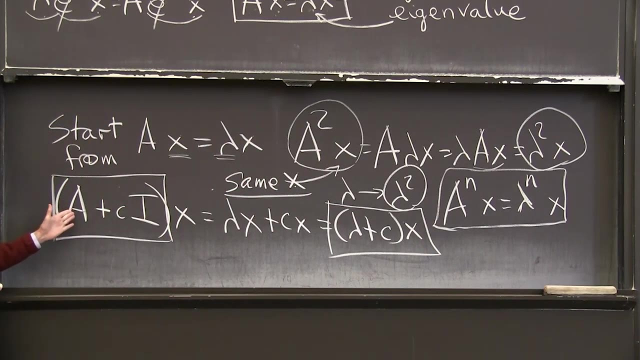 I've seen that the eigenvalue is lambda plus C, So there is The eigenvalues, for when I think about this as shifting A by a multiple of the identity, Shifting A, adding 5 times the identity to it, If I add 5 times the identity to any matrix, 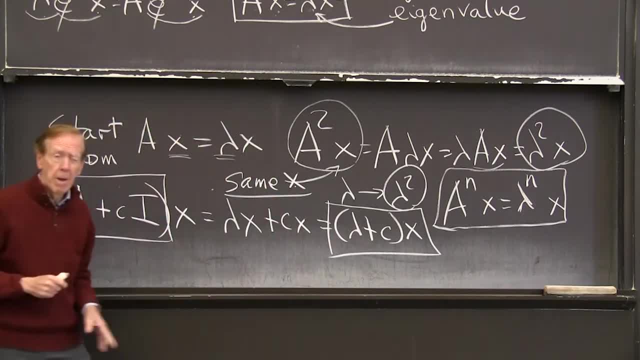 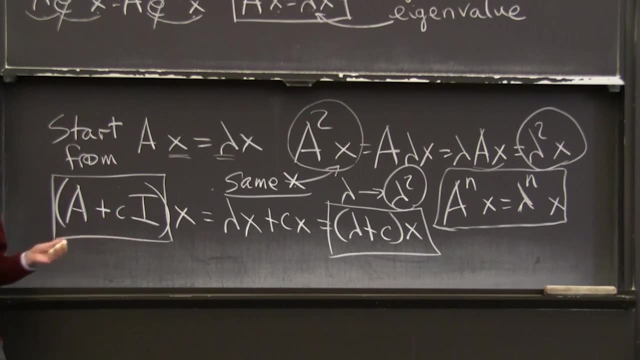 the eigenvalues of that matrix go up by 5. And the eigenvectors stay the same. So For As long as I keep working with that one matrix A, taking powers, adding multiples of the identity in the later, taking exponentials, whatever I do, 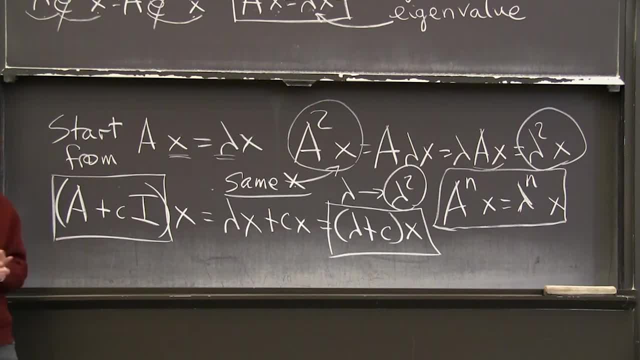 I keep the same eigenvectors And everything is easy. But don't think if I had two matrices, A and B, with different eigenvectors, Then I don't know what the eigenvectors of A plus B would be. 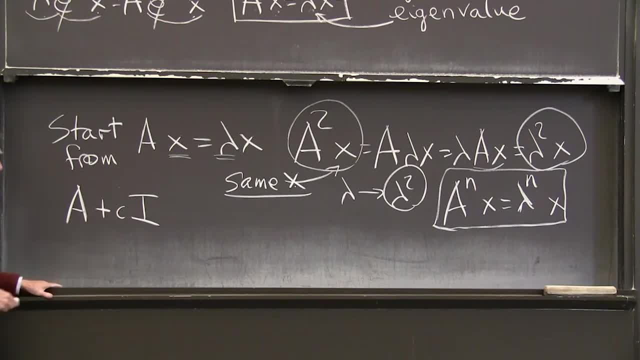 Two times the identity, Seven times the identity. And I want to know what about its eigenvectors? And the answer is same, Same x's Same x. I show that by figuring out what I have here. This is Ax, which is lambda x. 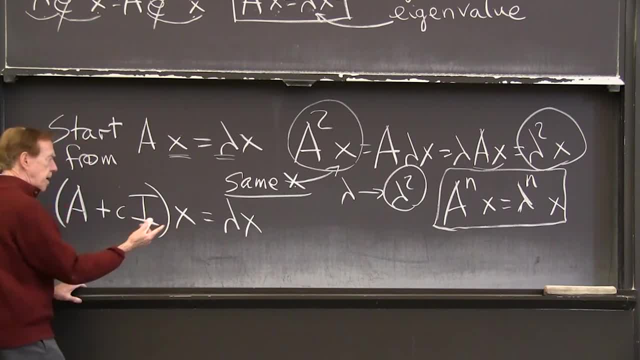 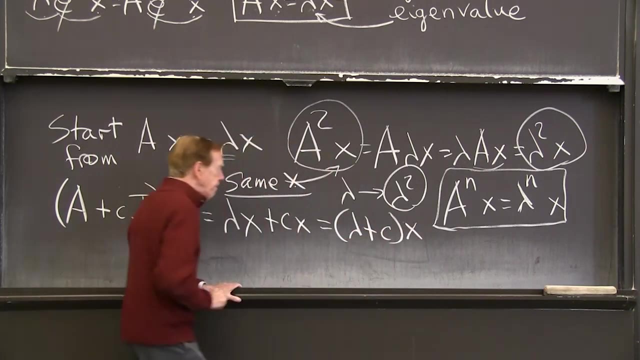 And this is c times. the identity times x. The identity doesn't do anything, so that's just cx. So what do I have now? I've seen that the eigenvalue is lambda plus c, So there is the eigenvalues. for when I think about this, 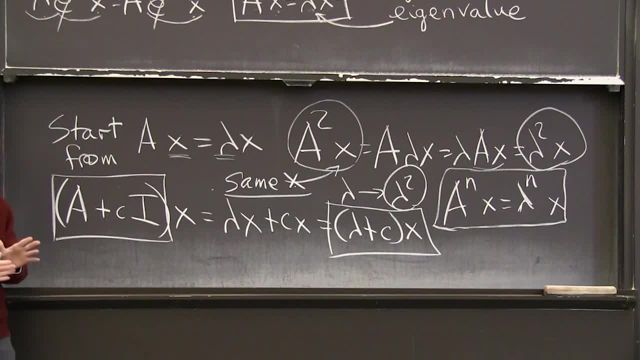 as shifting A by a multiple of the identity, Shifting A adding 5 times the identity to it. If I add 5 times the identity to any matrix, the eigenvalues of that matrix go up by 5. And the eigenvectors stay the same. 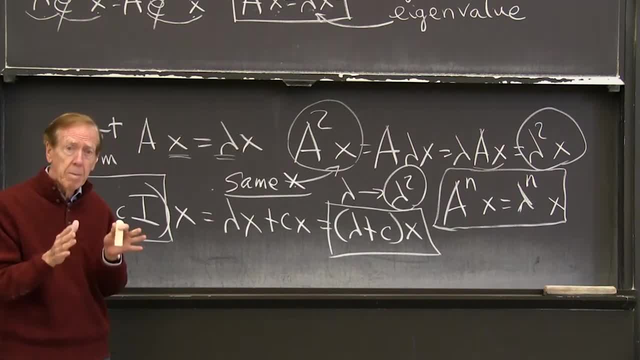 So as long as I keep working with that one matrix, A, taking powers, adding multiples of the identity in the later, taking exponentials, whatever I do, I keep the same eigenvectors And everything is easy. But don't think if I had two matrices, A and B. 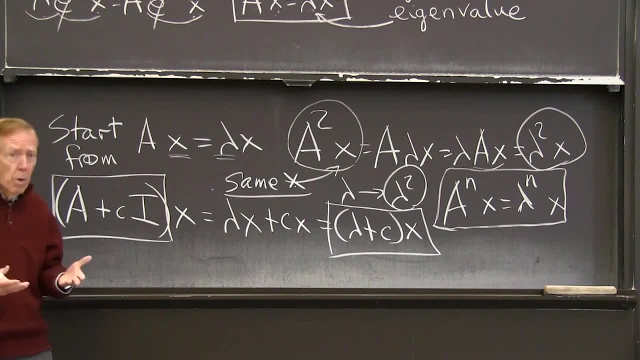 with different eigenvectors, Then I don't know what the eigenvectors of A plus B would be. I don't know those. I can't tell the eigenvectors of A times B, Because A has its own little eigenvectors. 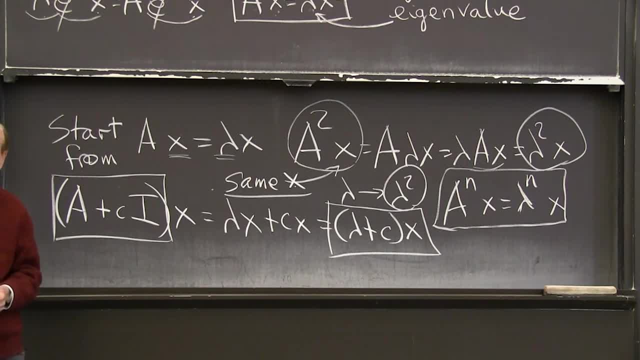 and B has its eigenvectors And unless they're the same, I can't easily combine A and B. But this shows what I. as long as I'm staying with one A and its powers And steps like that, no problem. 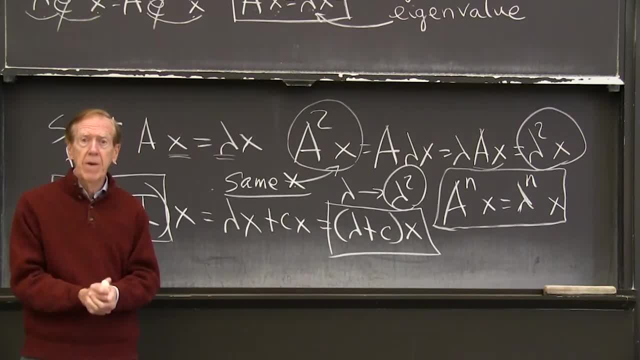 OK, I'll stop there for a first look at eigenvalues and eigenvectors.